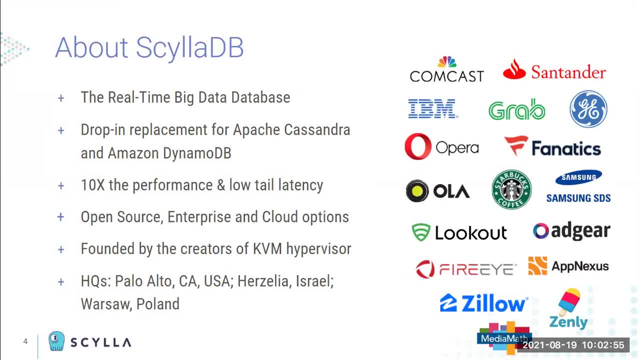 the database, the project, if you will, Scylla is a high-performance big data database compatible with Apache, Cassandra in the CQA level and compatible with Amazon DynamoDB, again in the API level. And by compatible I mean the compatibility in the protocol level. 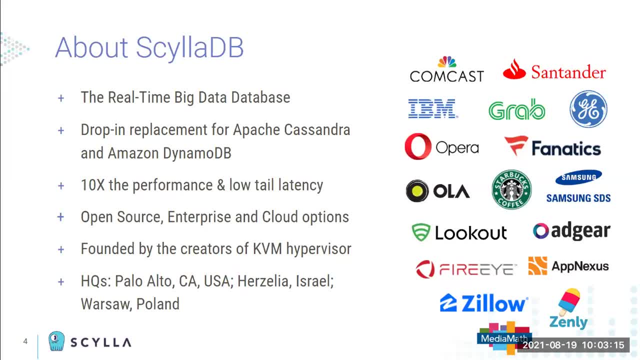 the binary protocol level, So any driver that works either with Cassandra or DynamoDB will work out of the box with Scylla as well, Although we have our own drivers that give you some extra boost for performance, but that's not in the scope of. 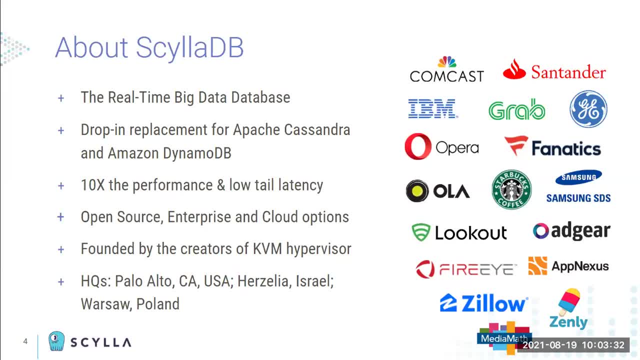 For this session. Scylla was developed with performance in mind. That's the P99 that I mentioned earlier. It was created in C++ with thread per core and a lot of goodies, a lot of focus on performance- Again out of scope for this session. You can use Scylla in three different 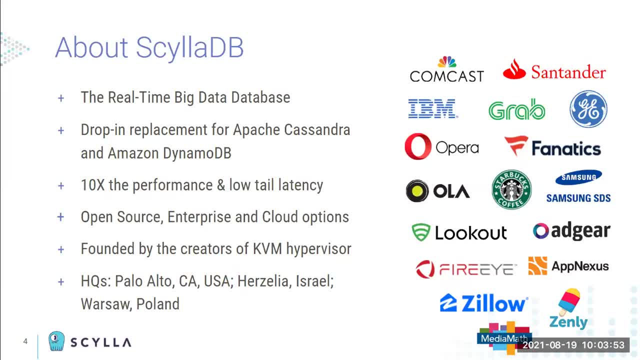 variants, if you will, although this word might sound scary these days, but that's a good variant. So the first is the open source. You can find Scylla in GitHub. download the code, compile it if you have some time on your hand, or download the binary RPM. 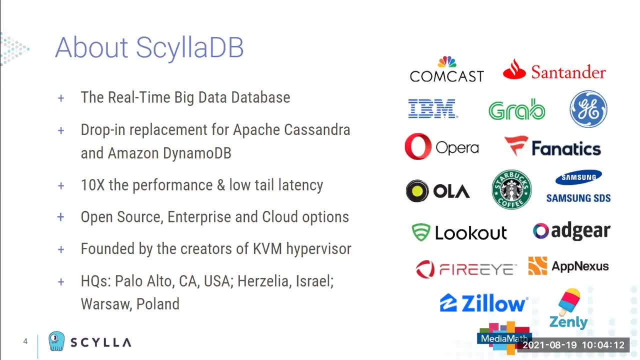 Docker You can find Scylla community AMI on AWS, on GCP and such. We also have an enterprise version which is based on open source, like 90,- I don't know, 95% is the same, but enterprise do. 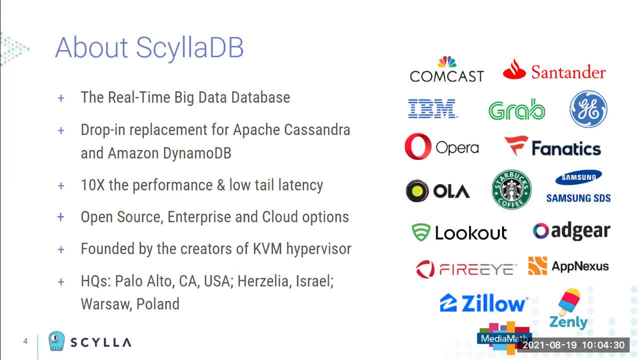 have some extra features, Mostly around security, but also around workload prioritization, and mostly enterprise is more stabilized, and that's the version that we provide commercial support for. And last but not least is Scylla Cloud. Scylla Cloud is a managed version of the enterprise. 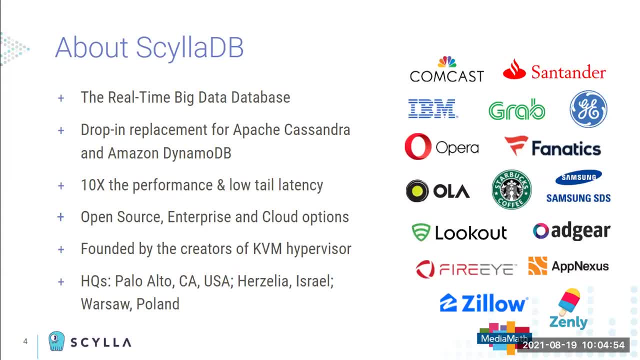 of Scylla Enterprise. you can consume it on AWS, you can consume it on GCP now And we are basically managing the cloud costs during the war. We have leverage of personal time. we're also managing the cluster for you doing upgrade, doing 24 by 7 proactive monitoring and everything that you. 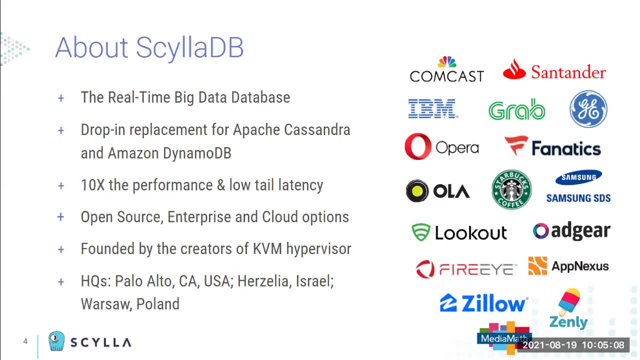 would expect from a database as a service these days. so check it out. that's probably the easiest way to take a Scylla for speed. so if you want to just test Scylla very quickly, the two easiest way i would assume is running Scylla as a docker or use Scylla and on the cloud and you don't even 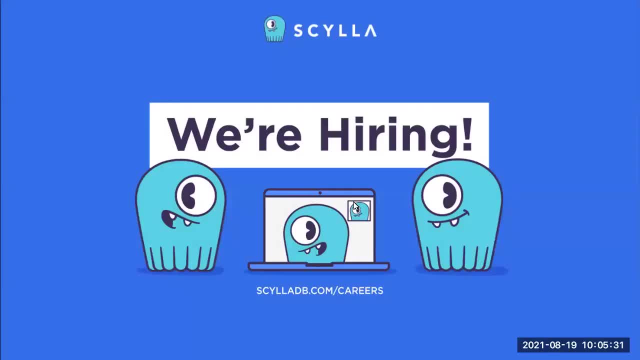 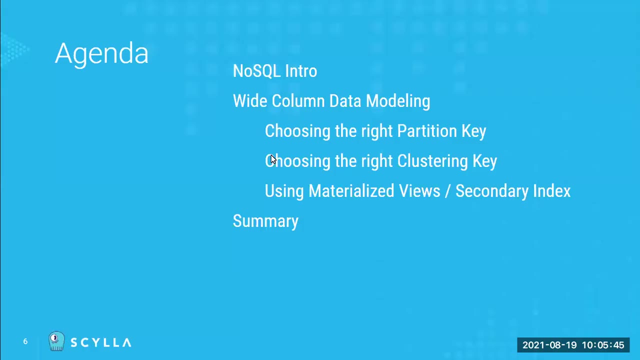 have to provide the credit card at first and we are hiring and with a lot of position, from developer advocate to developer in Golan with C++ and many other things. so check out our page. and so today's session is about the NoSQL modeling. so first, the first few minutes will 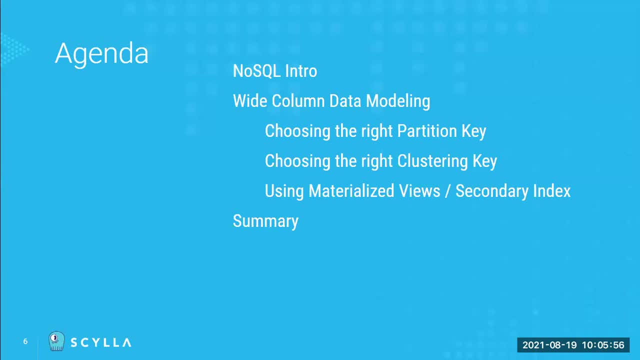 be about? what is NoSQL- although i'm sure the term is familiar by everyone by now, and but i will try to make it a quick and focus on Scylla. and then we're going to deep dive, or at least dive into wide column data modeling, partition, key, clustering, key, what this term means, why you. 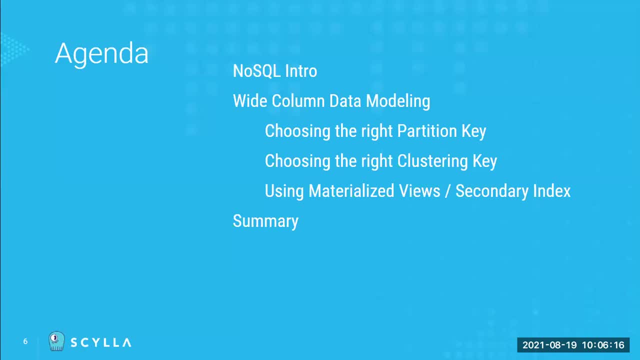 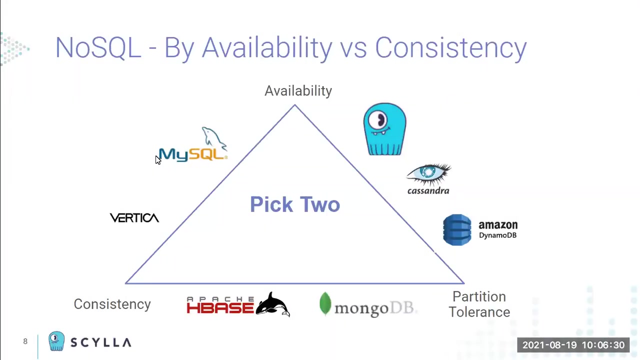 should be careful in choosing them, and we're going to explain what is materials doing? secondary index in the scope of NoSQL and Scylla, and then a quick summary and i'm sure we'll have some time for a Q&A. so what is NoSQL? NoSQL has been around for probably more than 15 years, and when people 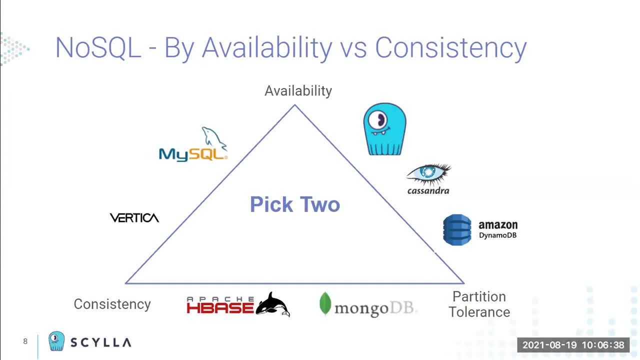 talk about NoSQL. they talk about a lot of things. it's a very wide term and there is- are probably hundreds of database that fit into the NoSQL title. there are a few ways to try to look at NoSQL from, i guess, two dimension. i don't know if you can see my hands from two dimensions, so 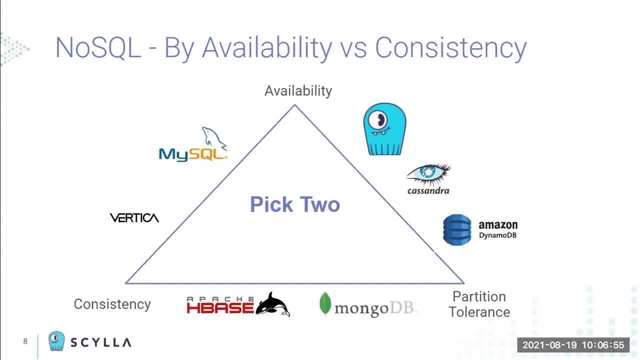 the first dimension is availability and you can try to partition all the databases, databases based on the CAP theory, for example. is it more consistent or is it more available These days? CAP theory considered to be old and not granular enough. There are more advanced category of that. 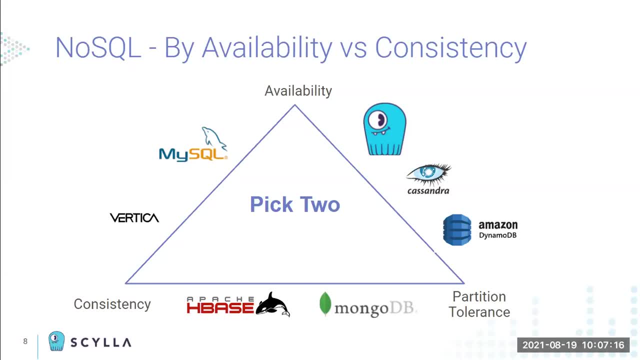 but on a very high level. Scylla, Cassandra, DynamoDB- all fall into the same category of eventual consistent. So, although there are slightly difference between these databases, the potential consistence described to some extent all of them, and in all of them you can actually do more granular. 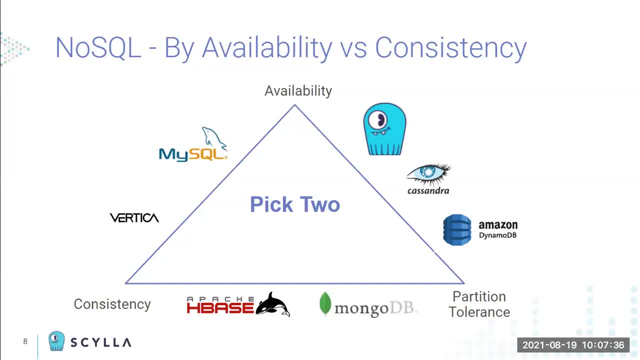 decision of what consistency level you want, But that's not the focus of this session, So let's leave it with that. By the way, if you are interested in this thing, you can check out the architecture pages on Scylla docs and also the Jepson reports in general. 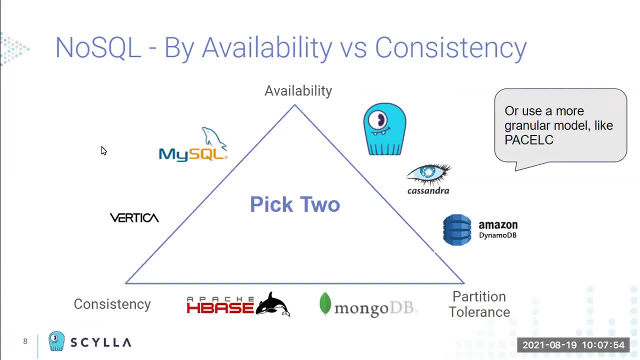 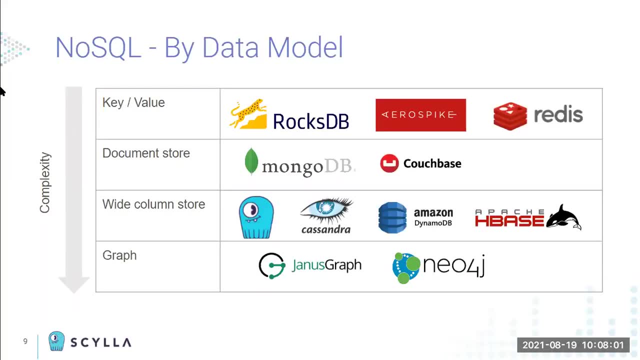 and, in particular, the Jepson report on Scylla, which go into this topic. It's a topic of availability versus consistency. Another way- that's the other way- access to categorize the NoSQL databases by data modeling, which is the focus of this session. 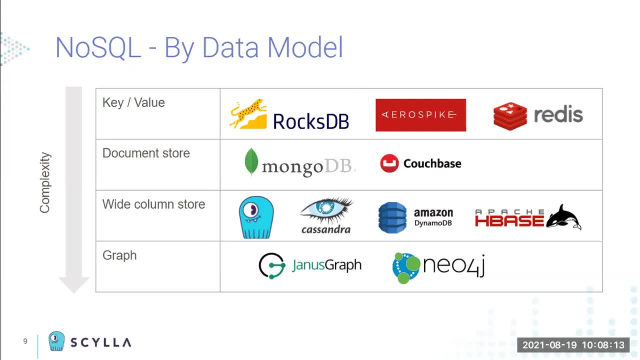 So I know, for people who are familiar with this database this seems to be crude, but so you can think of NoSQL database from the simple to the complex: data modeling. So the simplest will be key value, where you have a key and a value, as the name suggests. 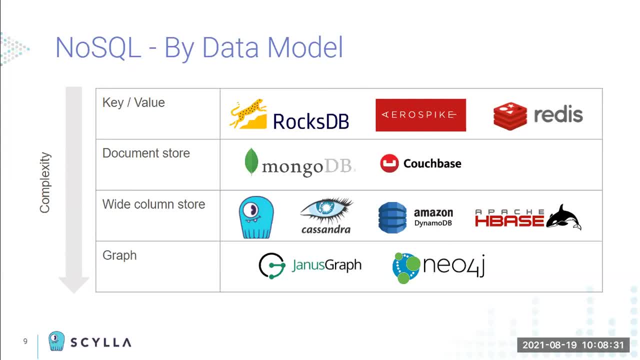 the value doesn't have to be an integer or one type. It can be a complex data structure depending on the database, And roughly you can put arrow spike in this category, Redis, which is a more of like an in-memory cache to this category. 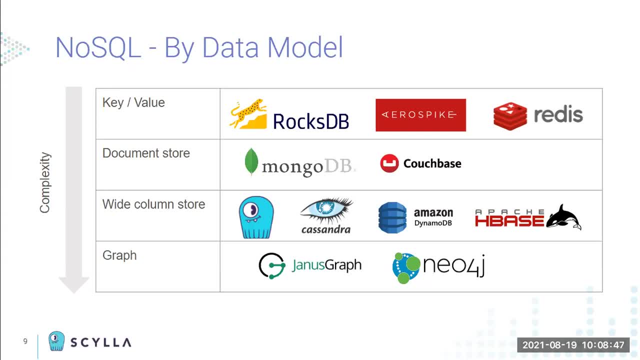 And I'm sure many are familiar with that. A similar data modeling is a document store- Document store- you can think about it as a key and a document as a value, And the document usually can be like a nested JSON or XML or whatever structure. 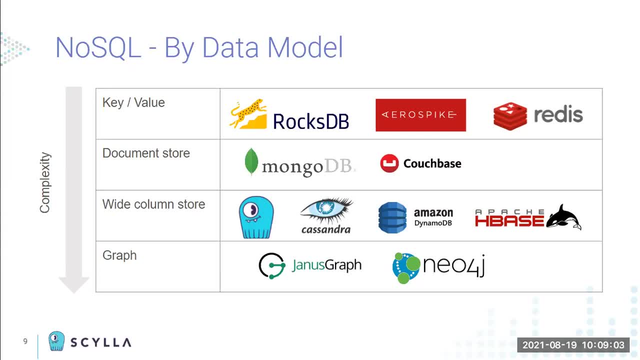 that you can look into. The third type, which will be the focus of this session, is wide column. At a very high level, wide column is a key, key value: The first key, partition key. second is clustering key and then the value. 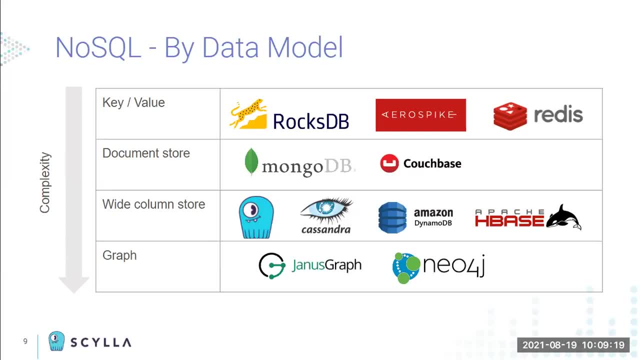 And we'll explain more about this data modeling at this session. And there are more type of NoSQL database, even more than than in this slide. there is graph database, GeoCeptal database, time series database and more and more. 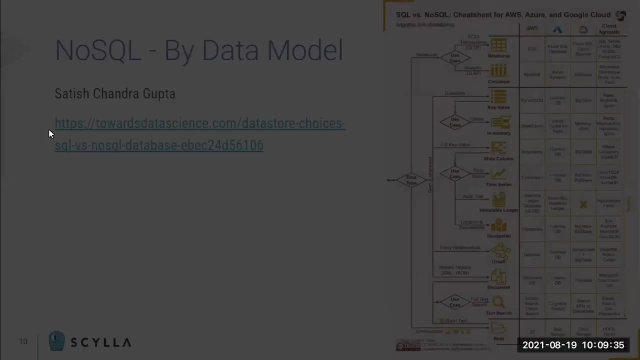 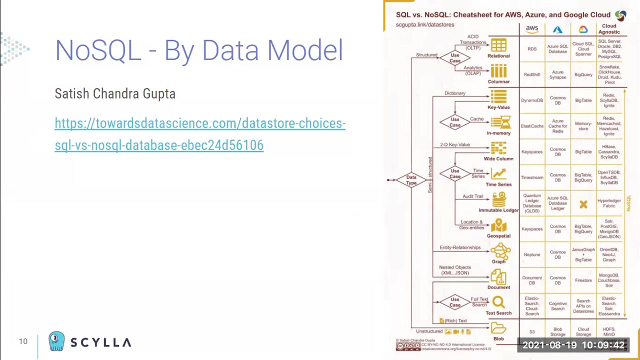 It's really an interesting and a very dynamic head of mail. I won't go into this diagram, but it's cool So I left the link in the slide, So if you get the slide later you can check it out. It's a guy named Satish, created like a graph. 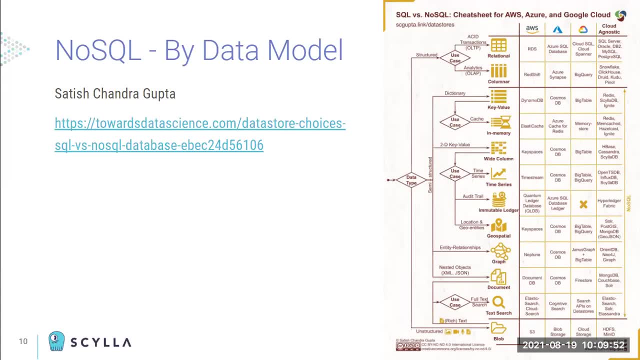 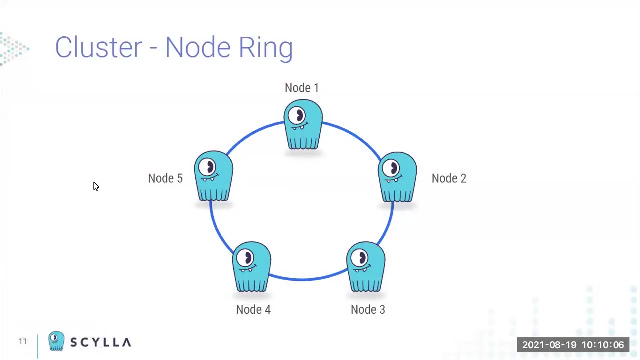 of most known database on all the cloud and off the cloud, And it's mentioned both Scylla, Redis and other databases that I mentioned in this session, So check it out. So let's start. when we talk about data modeling, the first thing to understand is that Scylla, 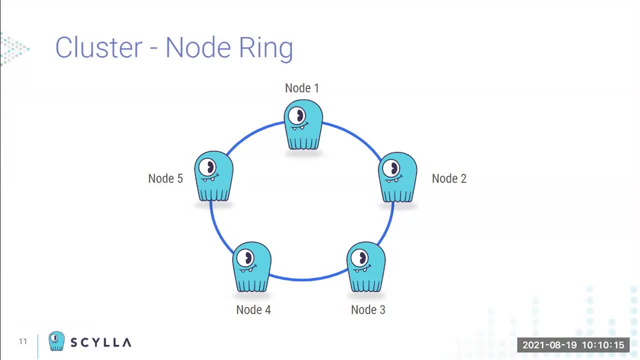 and most of the NoSQL databases are distributed databases. Distributed means that it's not all in one machine, It's distributed between many machine codes, nodes or server. I will put that in the description. I will call it node in this scope. So Scylla can support cluster from a three node cluster. 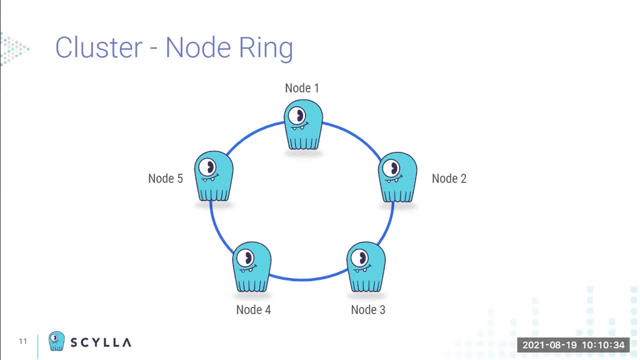 to many, many hundreds of clusters- sorry, hundreds of nodes in a cluster, separate to data center and reps and such. And the fact that the database or the data is distributed already set the first and most important data modeling aspect of it, which is the partition. 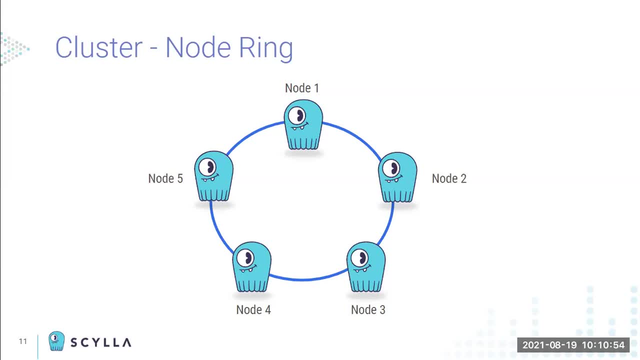 You cannot put all of your data on the same node, or even three nodes, because it just, if we're talking about many, many terabytes of data, it will not, just it will not fit there. So you're doing some kind of partitioning. 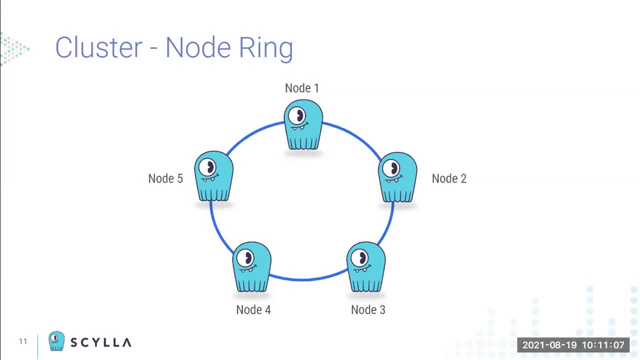 In the old days, or still today actually. if you're using databases like MySQL, you have to do the partitioning yourself, and with more distributed by nature database like Scylla, you don't have to do that. The database will partition that for you. 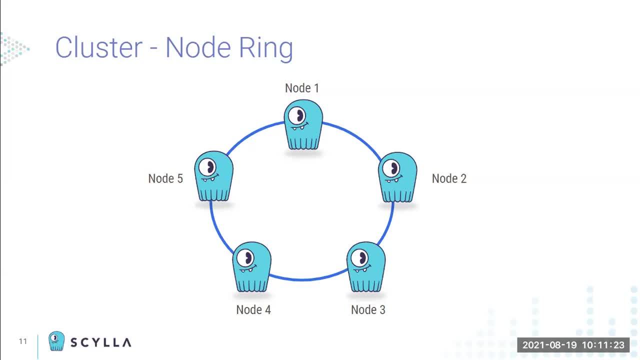 and it will do it using some kind of hash function. It will mention later In practice Scylla and other NoSQL database, not just partition data between the nodes, they also replicate the data between the node. The often people use application factor of three. 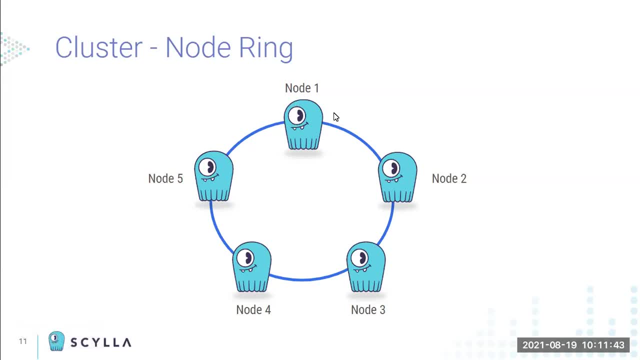 meaning that every information element will replicate, for example, a node one, two, three or another information element, or node two, three, four et cetera, and if you have hundreds of nodes, you can imagine it will be evenly distributed. 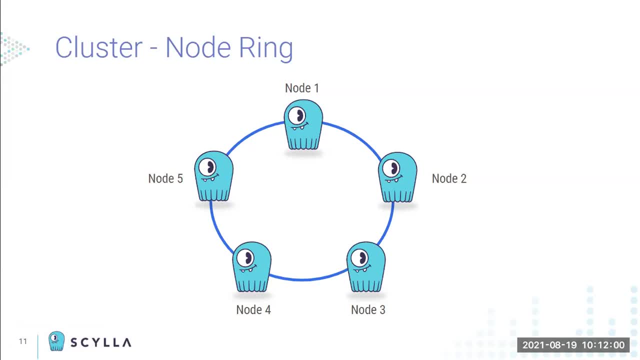 What I want to mention is, even though the data is replica, still not every node hold all the data. Still there are only three nodes- or four nodes, depending on your application factor- hold the information. So the database need to manage which information elements fit in each node. 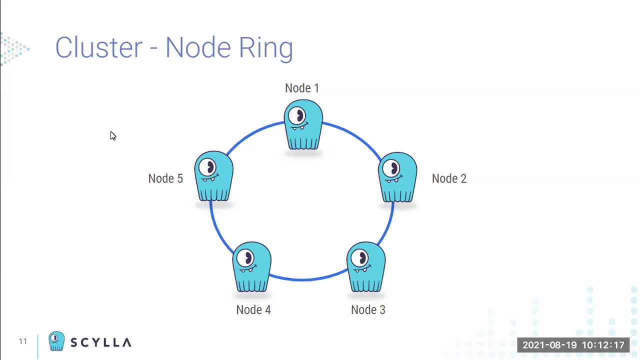 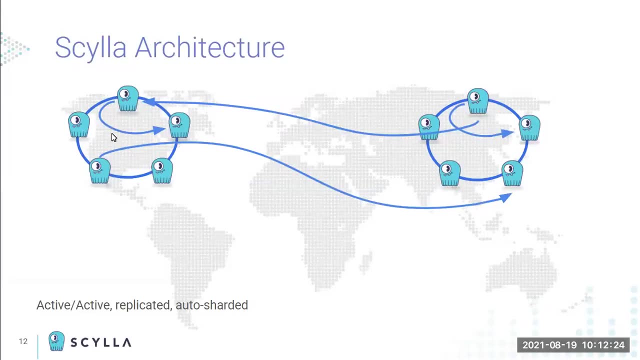 and that is the partitioning. That's the partition key, which is the first data modeling aspect that we're going to touch. Scylla, as mentioned, can also support multiple data center configuration. Data center usually mean a region, AWS region. 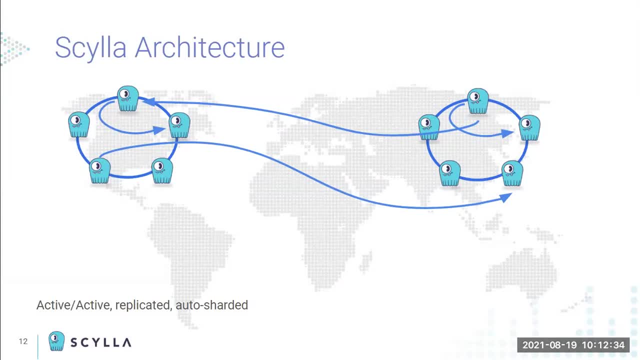 or GCP region or your own on-prem region, And the data is replicated completely offline in an asynchronic way. So it's very efficient. For example, you can have- usually you have application distributed as well, So the application, for example, in Virginia. 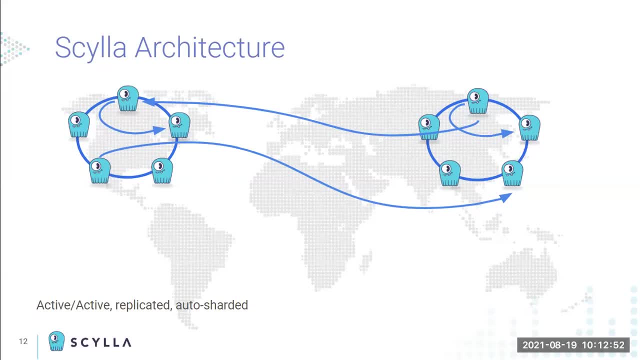 can query the data center on Virginia and the application running in Frankfurt can query the data center origin in Frankfurt, And updates are going in both ways asynchronically. So all the cluster, the two data center, are eventually synchronized. Usually it's take a few milliseconds to cross the ocean. 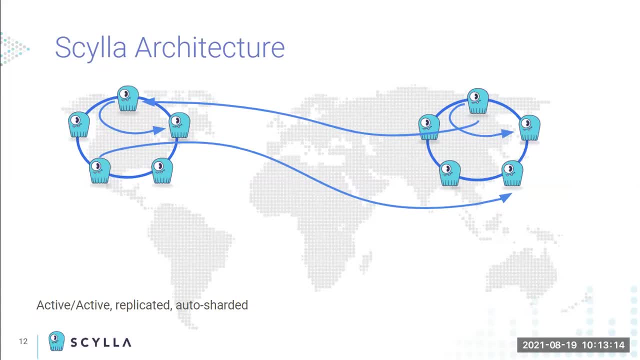 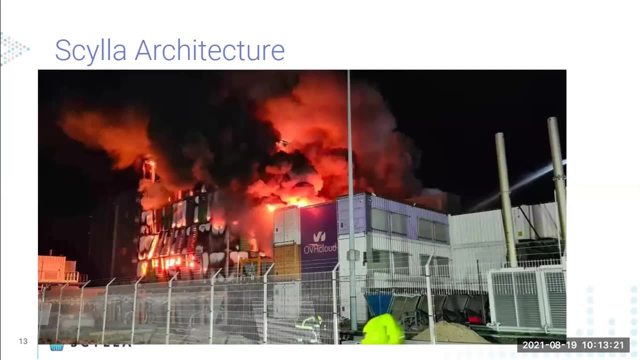 and maybe a hundred millisecond, And you can work in such a distributed way. This kind of architecture actually was recently tested by FHIR And for those of you are familiar with the OVH cloud, you know that one of their data center caught fire from some reason, I think a year ago or so. 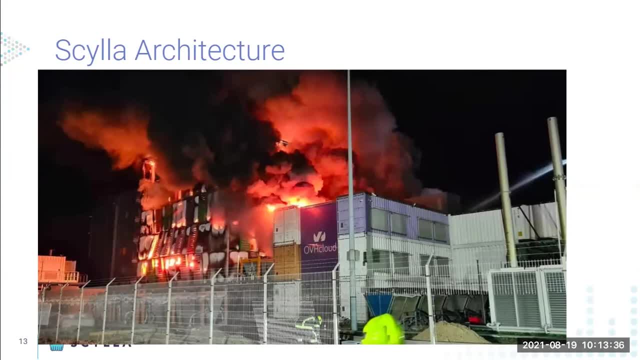 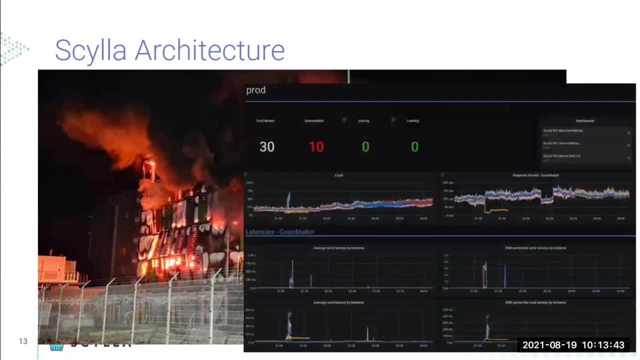 And we actually had a customer that was using this data center as one- luckily one of his data center in the Scylla deployment- And actually Scylla, as you can see here. that's a capture from the monitoring. So Scylla continued to function as expected. 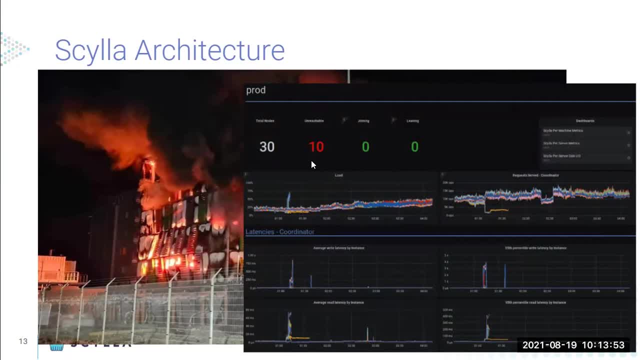 With a third. we have 30 nodes, 10 of them in this data center. 10 of the nodes went down, but the other nodes continue running as expected. So that was a really a trial by fire, if you will, of this architecture. 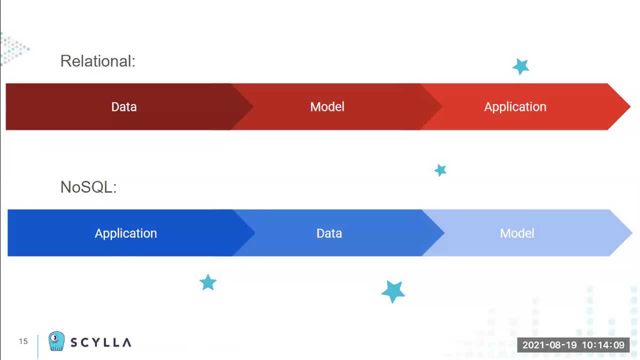 So when we're talking about data modeling- and this is like a generalization, but bear with me- So usually when we talk people on this call coming from SQL background, what they usually do, the process is: take your data, try to understand it. 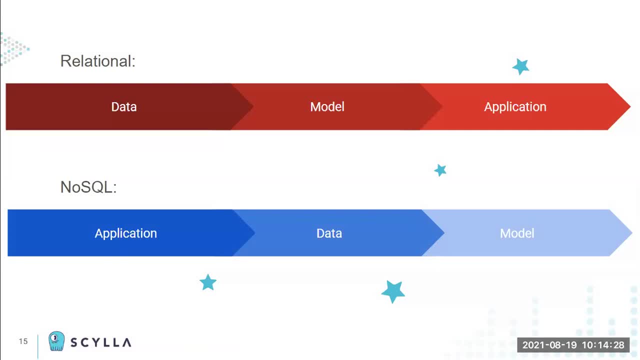 break it into element or entities- like people, offices, managers and such- understand the relation between this entity and create a table per entity with relations- And the relation could be a foreign queue, another table and such, And that's basically what you do. 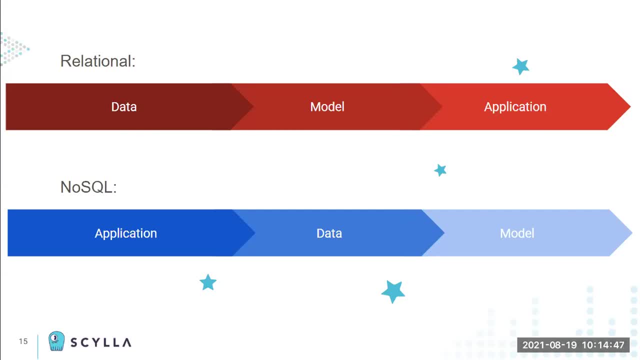 And you assume that if you have a good data modeling, your application can adjust, use it and it doesn't really matter what application you are using. You are modeling the data, not necessarily the application. On NoSQL, NoSQL in general. 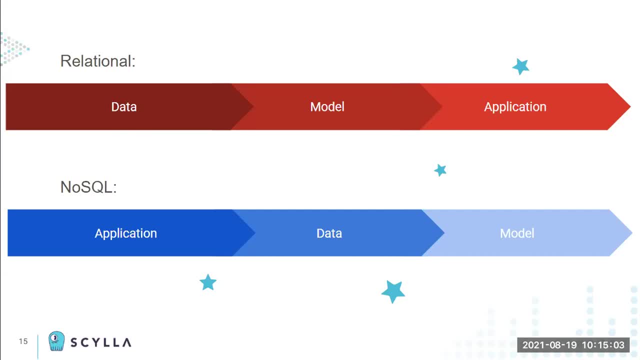 have a more limited data modeling, and that's true for all of the or most of the NoSQL database. They don't have the full power of SQL and they give up some fit in favor of availability, performance and other terms. 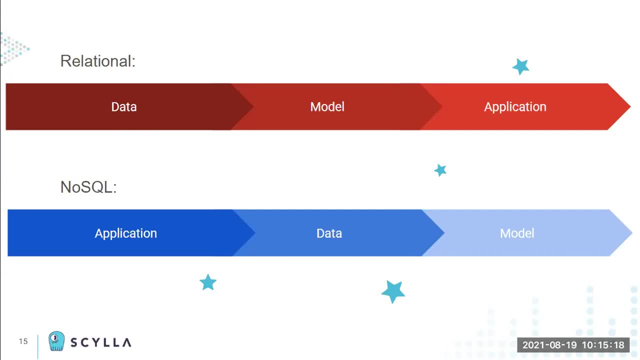 So usually in NoSQL, what you would do, you will write down, you will write down. you will write down exactly what query your application need to use and create your entire schema based on that and not the other way around. 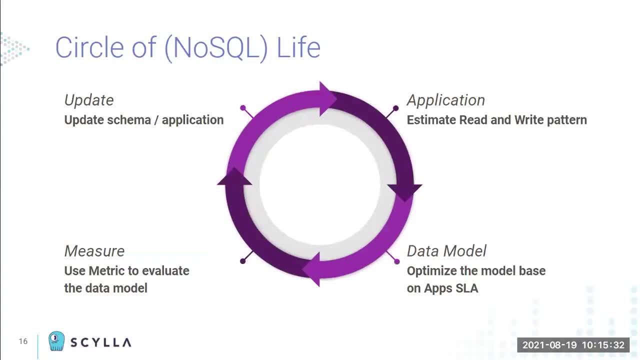 And that's what we're going to demonstrate in this session. One thing I want to mention that keep in mind, it's an iterative process. So, yes, you do write your, you do write your query and your schema and you assume it's going to do fine. 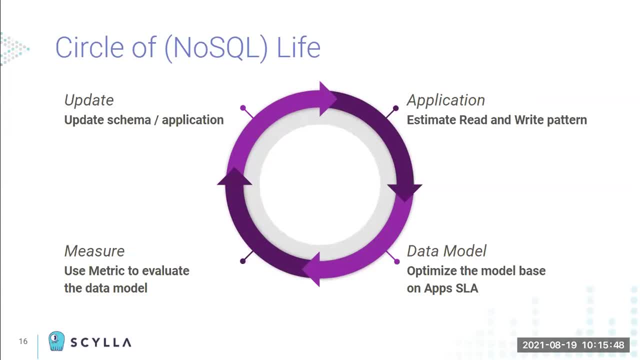 Hopefully you test it as well and even performance tests before production. but after, after a month, a year of production, a data pattern change, volume change, application change, at some point your assumption will break and you have to change the schema. 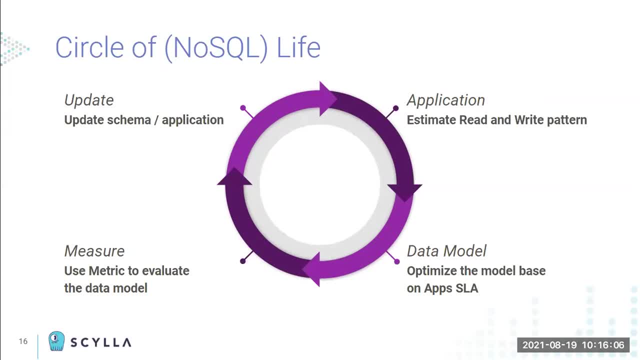 So it's- and that's roughly true for SQL as well, but even more for NoSQL, because you have to take more assumption. So keep in mind it's an iterative process. It's a never ending process of creating a schema. 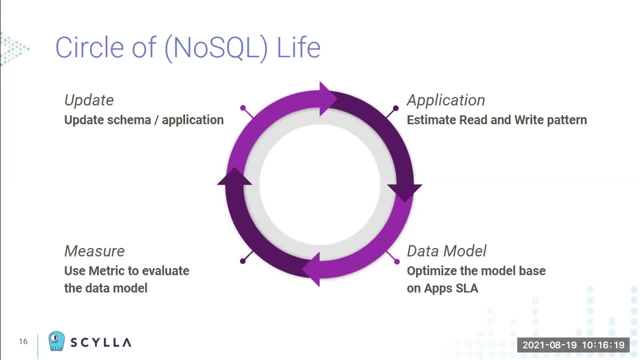 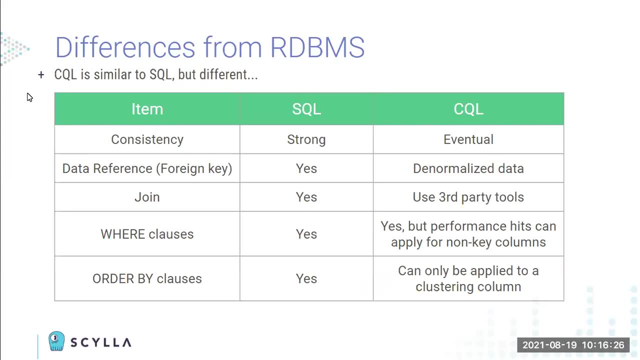 populating the data, continue monitoring, monitoring, monitoring, monitoring and at some point you probably have to change your schema, And so some of the differences between SQL and NoSQL, and again that there are many, many variants to it. 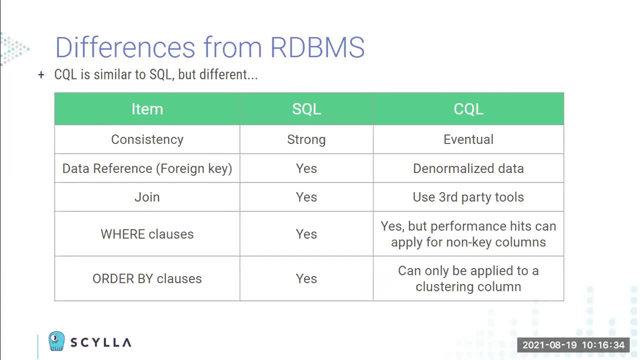 Each NoSQL database have slightly different approach. So just an introduction. So NoSQL database, or actually here, when you see CQL- for those of you who aren't familiar with the CQL is the Cassandra Query language. This is what Scylla use. 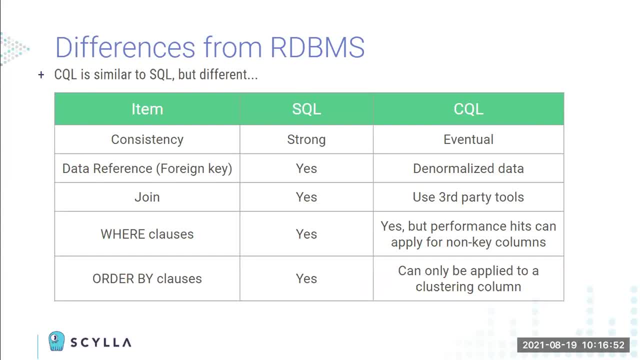 In most cases, And so you can think about it as a NoSQL in this scope, And so the data is de-normalized, you don't have joins, you don't have nested where you have limited order and such, but we do have way to bypass all of this limitation. 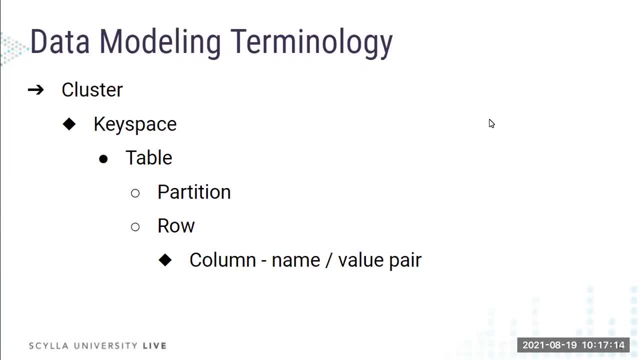 to some extent and we're gonna talk about it shortly. So the data modeling is some terminology for data modeling And in Scylla. so the cluster we mentioned, the cluster is actual nodes. Then you have a key space. A key space is like a database in SQL. 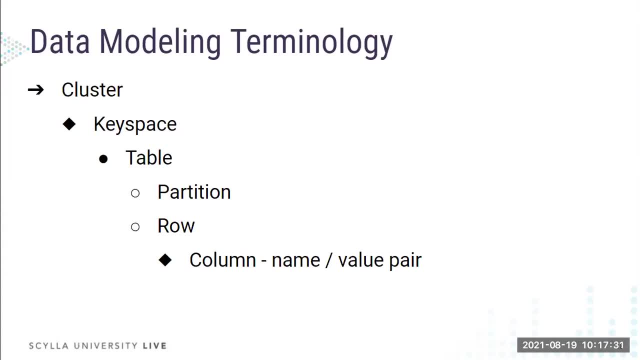 It's like a collection of table. You can think about it as a collection of table. Key space do have some properties that we're not gonna cover in this session, but some of this property are an application factor, use of defined types or the defined function in some cases. then another term. 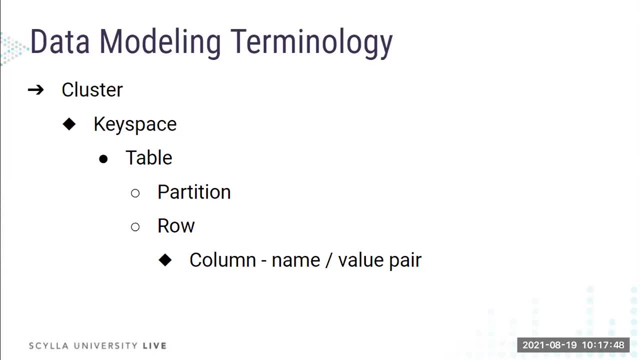 The second term which should should be familiar for people coming from SQL as well, is a table. A table- you can think about it again, I'm demonstrating it with my hand- It's. you can think about it as a matrix of columns and rows. 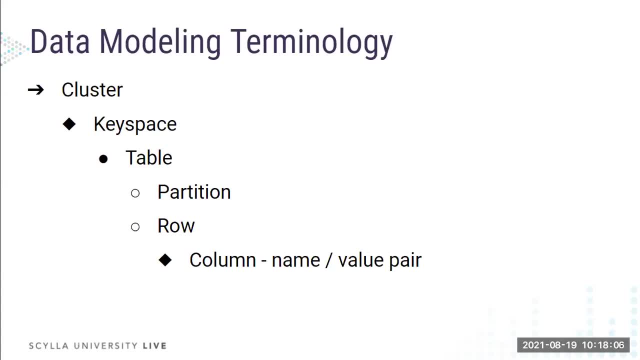 and each cell holds some information or it's a record, So each cell can be one field, can be a collection and such. So so far it's pretty similar to SQL. The difference here is the partition, and that's what I mentioned earlier. 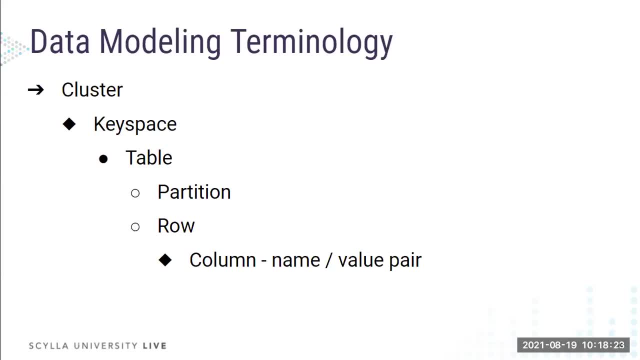 We have to somehow partition the row and the table, two servers, those two nodes, And the partition is a collection of rows, if you will, all placed on the same place, on the same physical node. So the first thing that you need to do 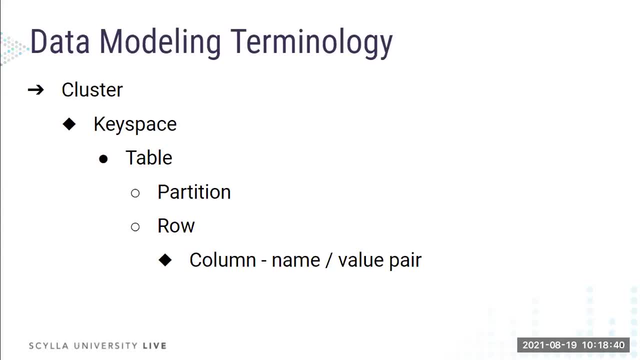 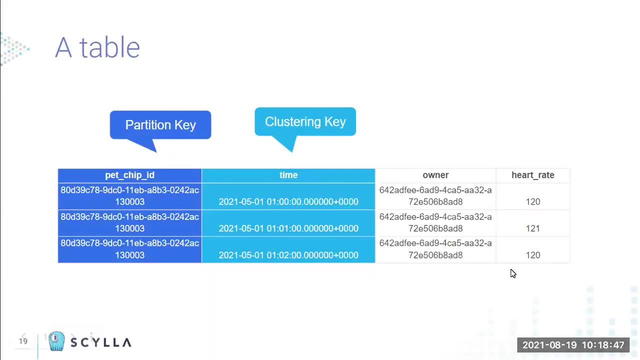 when you define the table in Scylla or Cassandra or DynamoDB, is defining what is your partition key, And that's the main concept here. So so here is a table. This table can be- I will explain this table later- but just the matrix that I mentioned earlier. 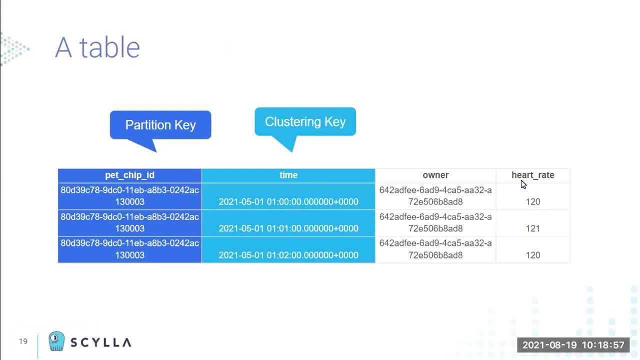 you have in this example. you have the pet ship ID, the time, the owner and the heart rate is the column, and these are the rows. Note here that some of the rows fit into the same partition, So that's what I mentioned earlier. 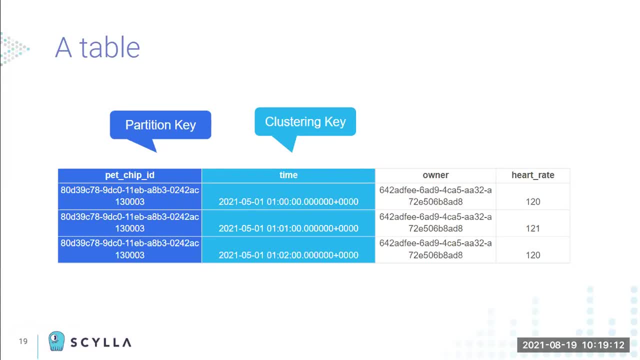 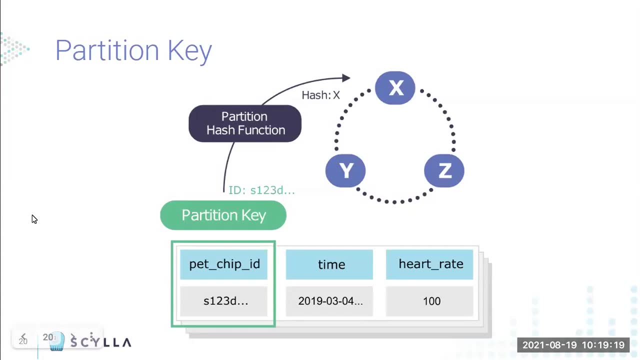 I'm going to don't need to read the fine details here. I'm going to continue with this example in the next few slides. So, partition key: as I mentioned, partition key is the most important function of the data modeling. A partition key: you define a collection of your column. 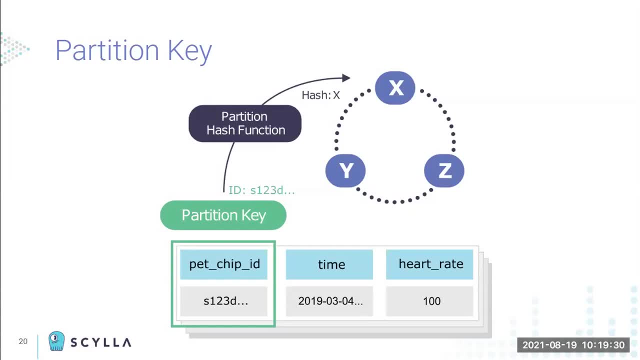 in your table as the partition key. In this case, in this example, the partition key is just the pet ship ID, but it can also be more than one column. There is a hash function in Scylla called partitioner. Let's take this key, hash it to a number and, using this key, 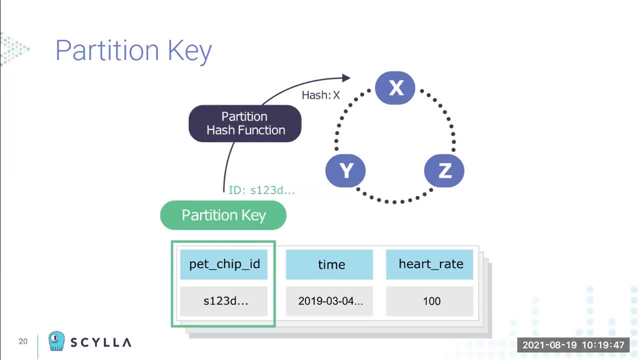 let's take this key, hash it to a number and, using this key, let's take this key, hash it to a number and, using this key, find which node should hold this data. And usually it's more than one, usually three nodes. 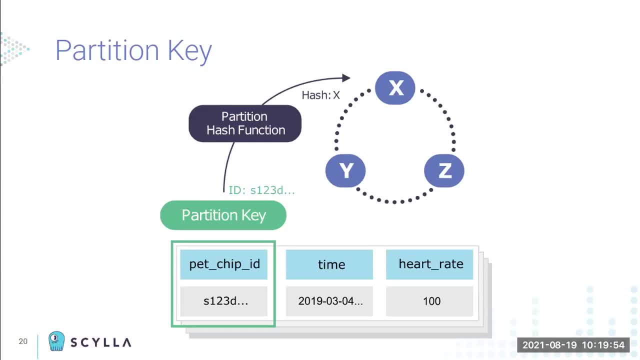 but the principal is the same: Each node in Scylla and Cassandra and similar database, each node called what is called a range of tokens, The entire cluster, lifespan of the token, rank and basically this function lets the database know which node in Scylla which, even which code, çevミ. 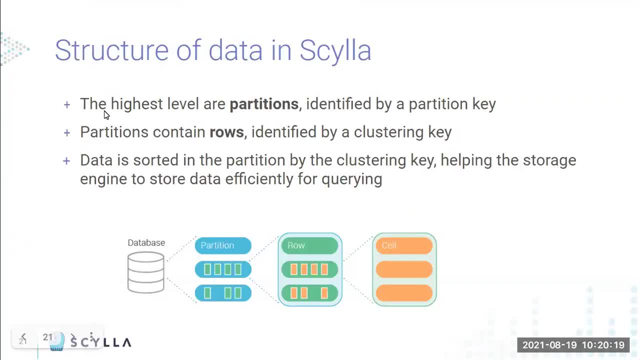 and so that's another diagram of the same principle. so database or key space, a whole table. if the table split into partition, where each partition is located on a specific subset of nodes, each partition composed of rows and each rows have cell, and the cell hold the actual information in 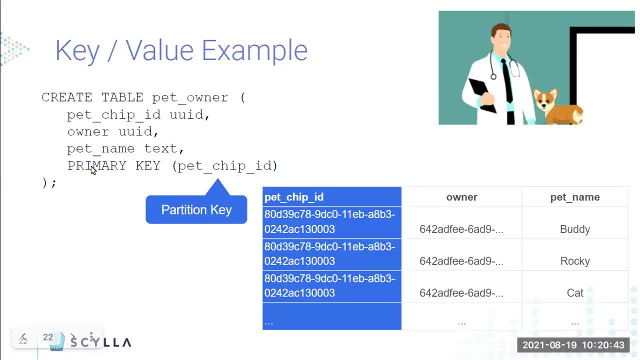 database. so so far, so good. i hope let's see an actual example, uh. so throughout this, uh, this session and demos, i'm going to use an example of a imaginary startup that collect information from colors of pets and the first table we're going to see. it's very simple: starting with the most 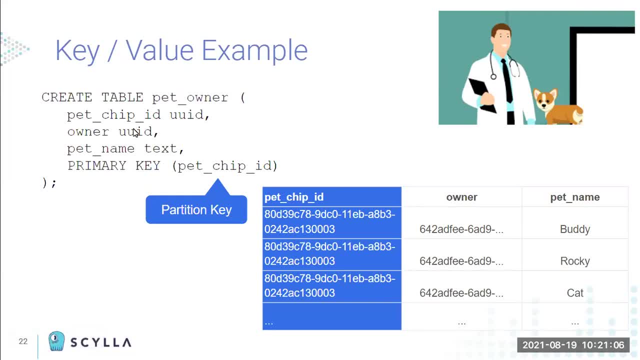 simple example. there is a pet ship id, owner id, the name of the pet and nothing more than that. so no additional data, sorry. and in this case we're using: and the pet ship id is a partition key. this is the syntax that we're using on cql, so that's an actual schema from cql. as you can see, it's pretty similar to. 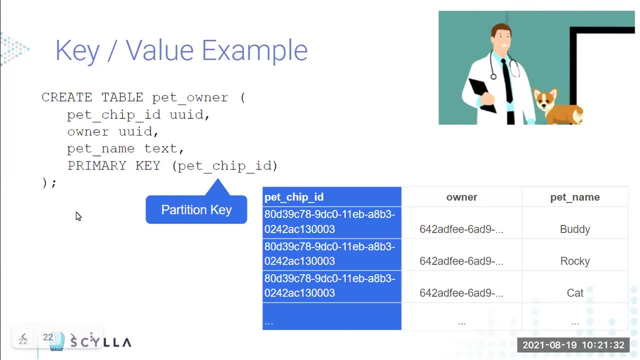 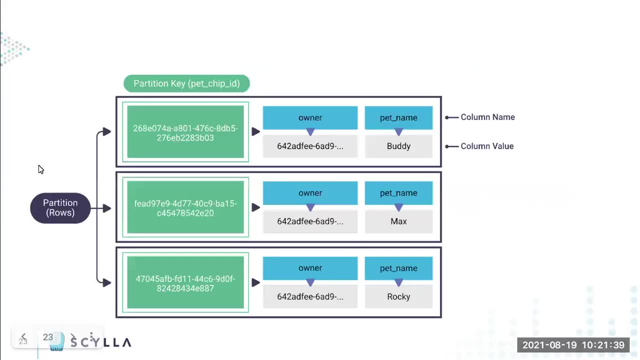 sql, but not exactly the same, and the fact that it's similar actually confused some people. so keep in mind, it's not sql, it's cql, and this is how this table will look like: uh, logically at least. uh, there is a partition key and the reason this example. 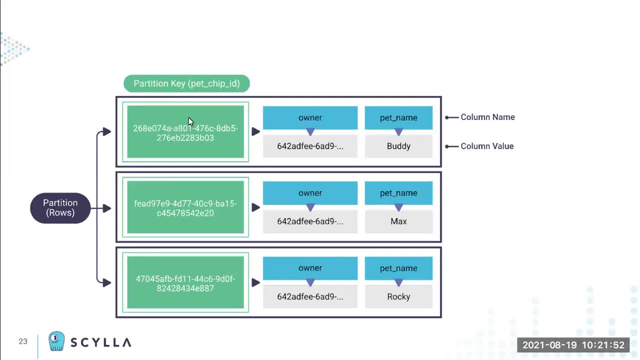 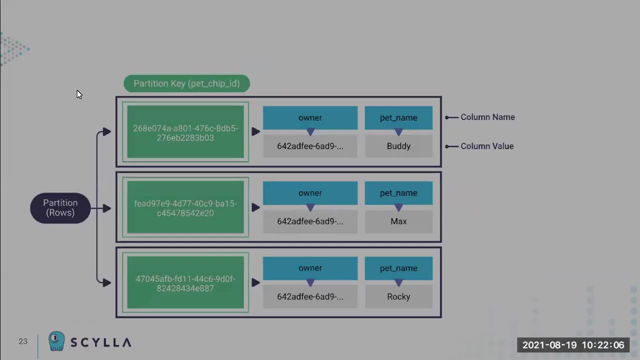 one. it's the most simple example: one row in each partition. so you can think about it as a key value use case, because we don't have a classroom key, we only have a partition key and a set of values, and later we're going to see a more complex example. so that's, that's a basic thing. and now, 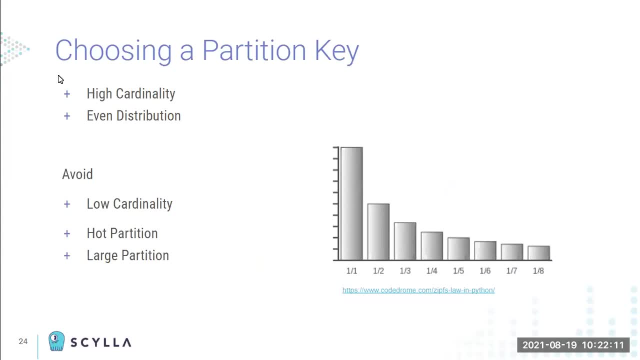 comes the question: what will be- and that's a key question, maybe the most important question in this, in this presentation- what will be a good partition key? because if you choose the wrong partition key, you are putting yourself in a bad situation from the start. so a good partition key have two properties: high cardinality and 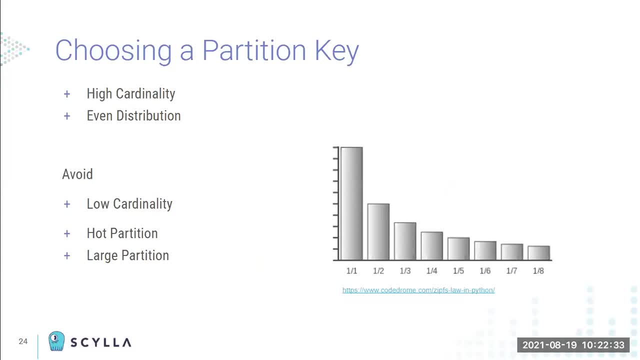 roughly even distribution. high cardinality is very simple. high cardinality is meaning: how many partition do you expect to have in the database? so sila can easily support billions- and i really mean billions- of partitioning in a database. so we want to choose a partition key that distribute this, this partition, across the nodes. so we want 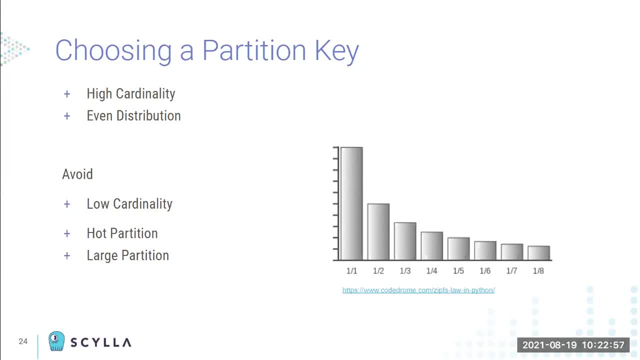 to choose the one with high cardinality, and we'll give example soon. the second is even distribution. you don't want the majority or a big chunk of your partition to be in one node. why? because you you are wasting resources. this node will be overloaded and the rest of the node will. 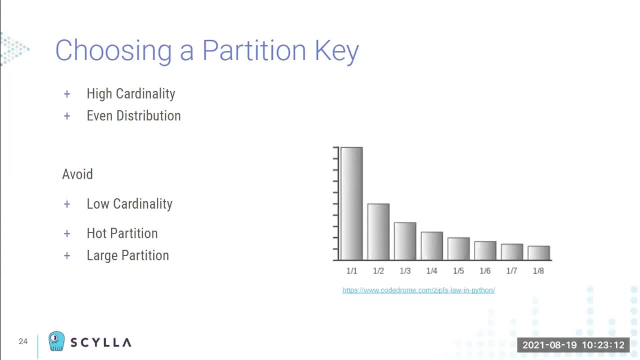 not do much. by the way, sila: in sila it's even more important than other databases because sila it's not, it's not a performance session, but in sila we did a lot of work of actually splitting the data and the computation inside each node to internal cores, where each core at cpu basically is handling a. 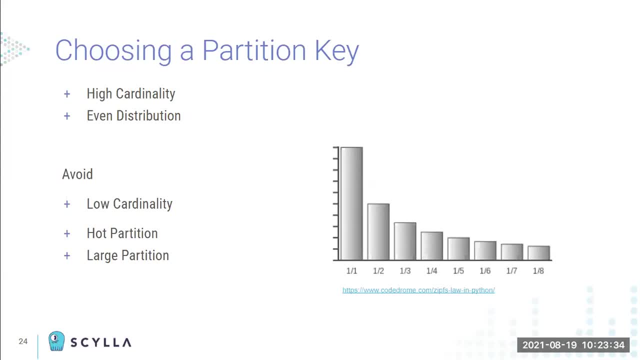 subset of the data. so if you have all the data falling to the same node and even to the same core, you are basically missing the new system and what? what will be a bad partition about partition would be a partition with a low cardinality. that's gonna lead to hot partition, large partition, and i will explain what each in a second. 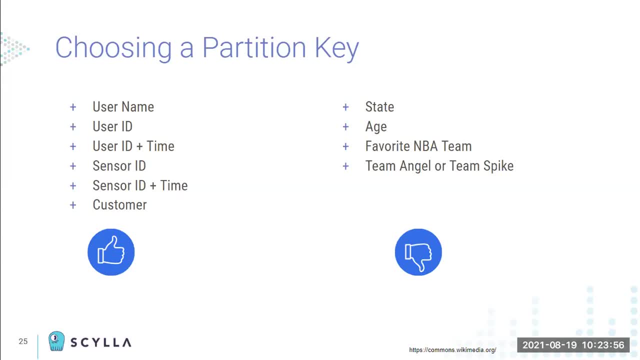 so a few example for bad and good partition keys. so classic example for a good partition could be a some kind of uuid or username or a customer name or customer id or something like that. A bad partition key will be anything that group the information to a limited number of. 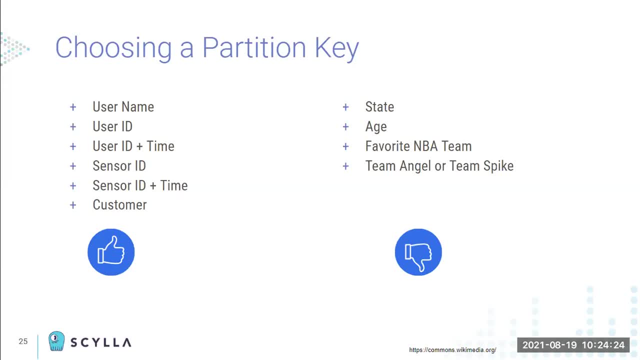 groups So it can be a state. it could be age or something like that. That would be bad partition. Why is it a bad partition key? So imagine that you have a partition key by state in the United States, So you only have 50 states, which can be already lower than the number of nodes that you 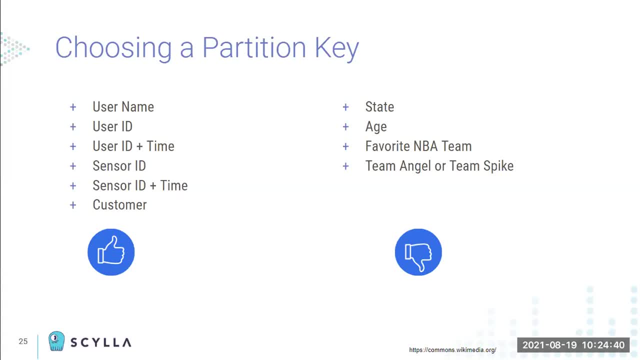 have on your cluster. So already it doesn't make a lot of sense, And not just that you can have many of you. for example, California is a relatively large state with a lot of people, So a lot and a lot of the input and output will be on the same node because you have a partition. 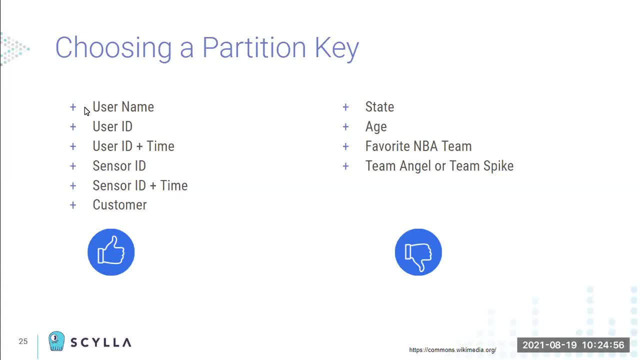 for California. It doesn't make sense. By the way, customer in some cases doesn't make sense either. It is depending on your data. You know your data better. So we had customers or users of Scylla. we chose something like a customer as a partition key initially, But after a while. 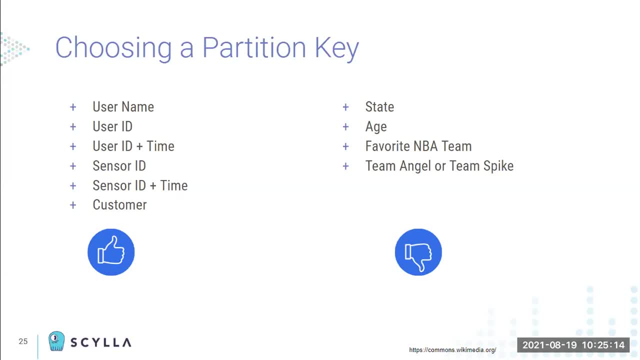 it's turned out that they don't have a huge number of customers, And not only that, they're very unevenly distributed, So 90% of their incoming traffic came from one customer. So using the customer in their case as a partition key didn't work well, and they have to change it. 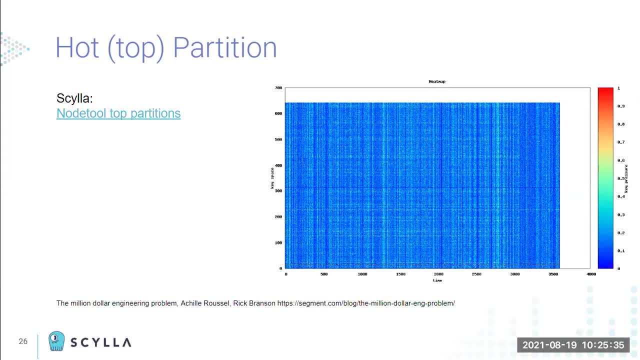 So what I already mentioned, what is the risk of traffic? Well, in the case of Scylla, the risk of traffic is the risk of traffic. So if you choose a bad partition key, or not just bad, it can start good and turn bad later. You. 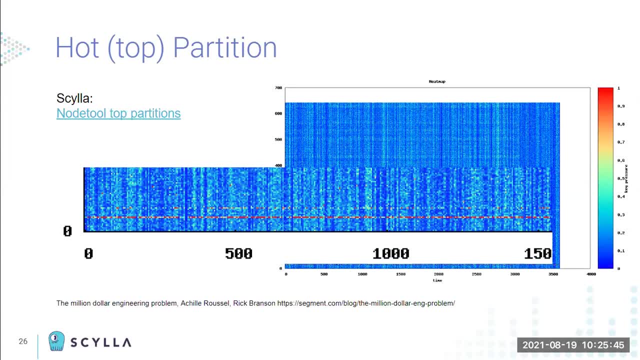 don't really know. And a hard partition is a case when a lot of the traffic hitting the same node in the same partition or the same core. And this is actually an example not from Scylla, it's an example from DynamoDB. All the NoSQL databases have this issue of a hard partition because 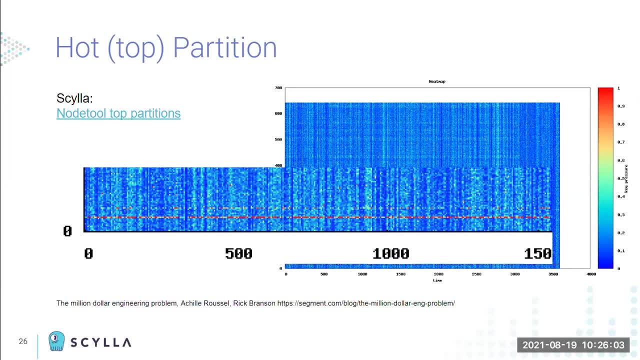 every time you will partition your data, the partition key might fail. So it's a common problem, And this is an example that they took from an interesting blog post. check it out. the Million Dollar Engineering Problem And I don't know if you can see it, there is a thin 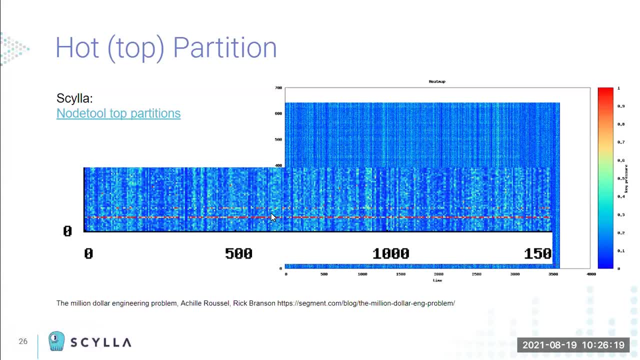 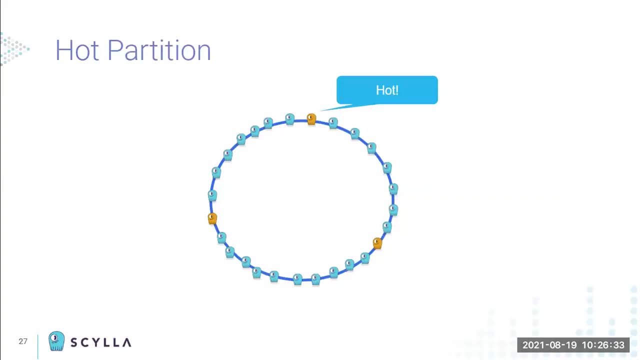 red line here that represent the hard partition. By the way, there is a movie- the thing with line, not related to the session but recommended in a way, Transmalik directed, But a little bit off topic. And so why is the hard partition is a bad? It's a bad thing, as I 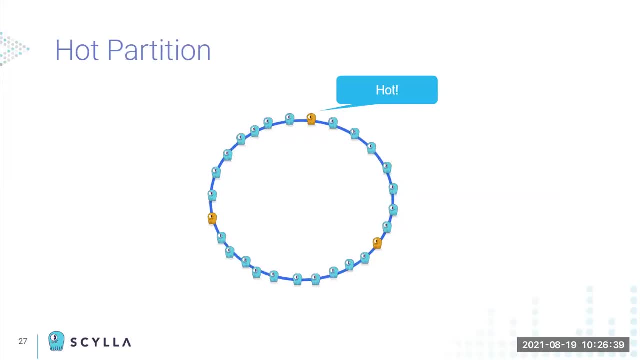 mentioned. Imagine that you have billions and billions of data, you want to support tens of million requests per second- which is very feasible in Scylla- and you invested and created a pretty large cluster of 30 nodes, But most of the traffic actually go to one node. So what will? 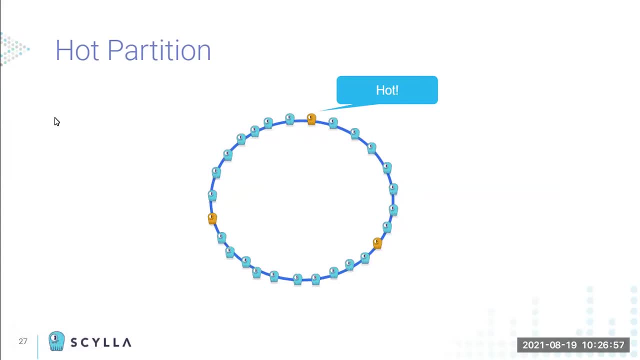 happen in practice, these three Scyllas, or three nodes, will be red hot and overloaded, So at some point they cannot even support the traffic that the user is sending, While all the other nodes are doing basically nothing or almost idle, or handling just 50% of the traffic. 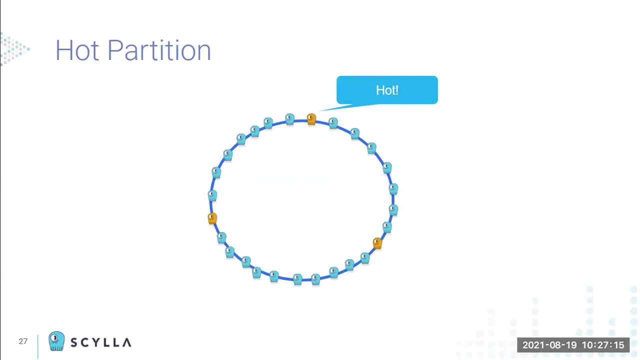 So you are getting. you're asking if you will, on two fronts: One, you invested a lot of money, but most of the nodes are idle. And second, the nodes that are loaded cannot handle the traffic, So you start getting all kinds of time. So that's the situation in a hard partition use case. 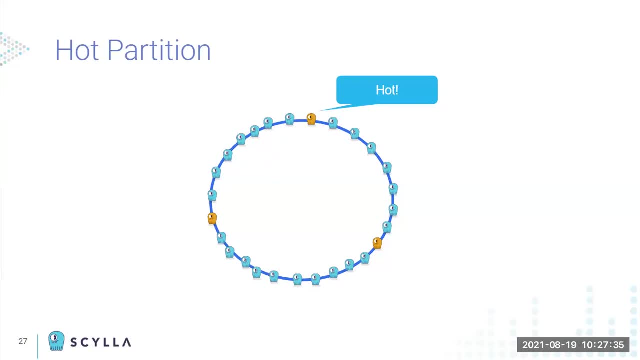 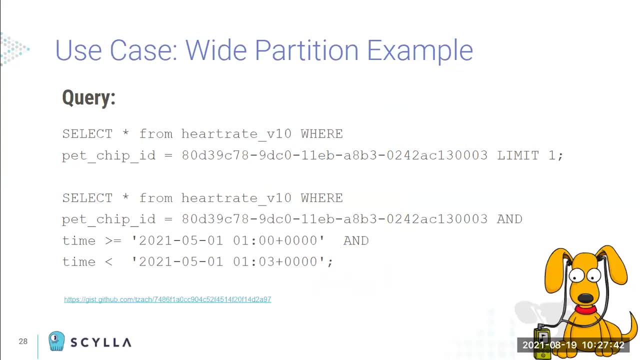 and you want to avoid it. First by selecting a good partition, second, by monitoring the system and validating. you are not hitting this case, And there are tools in Scylla that allow you to do that. Okay, so I'm done with the key value use case and explaining. 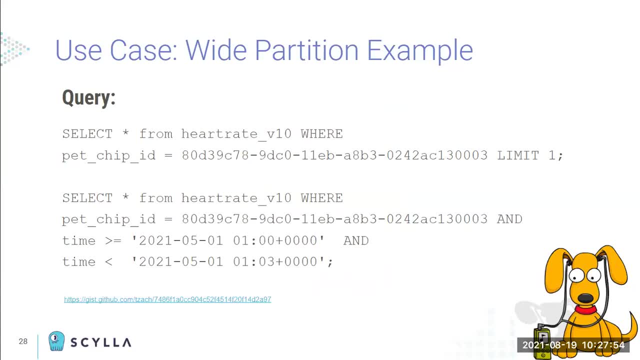 what is a good partition key? Second, I'm going to talk about wide partition because, as I mentioned, Scylla is not just a key value. it's a key key value: data modeling. So always starting with the query. So let's imagine that you have a data model and you want to start with a query, So let's imagine: 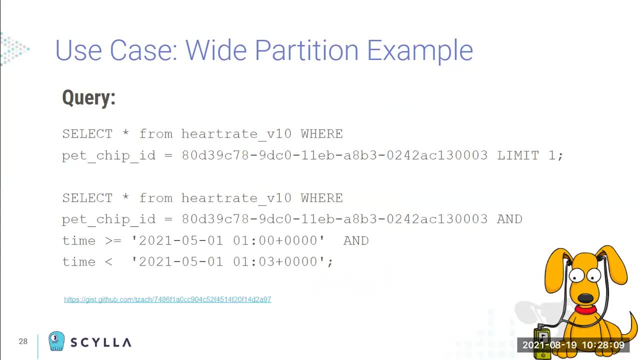 I'm going back to the same example, but in this example I have an application that actually collects information from the pets and reports it back to a database. Imagine an application that every second records the heartbeat, the I don't know the number of steps or what's not, of the pet and set it back to a database. and you want to do. 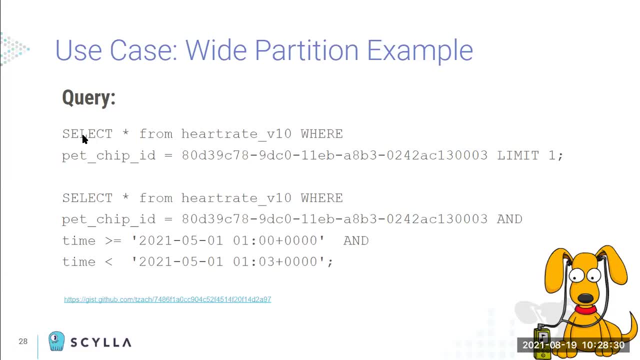 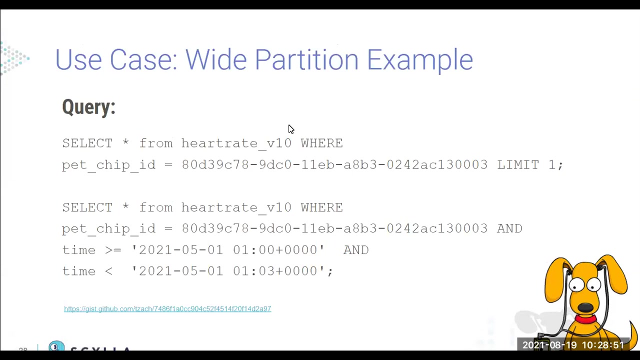 query like the one mentioned here. So, for example, select the last heartbeat for a specific pet or specific dog, or even more than that. that's a slightly more complex: select all the heartbeat of a specific dog but a second of a specific dog between in a time range, So between this time. 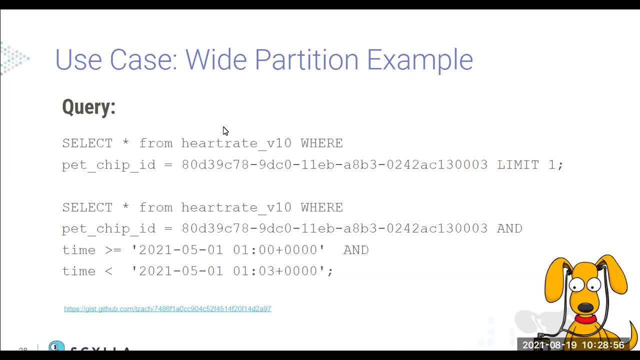 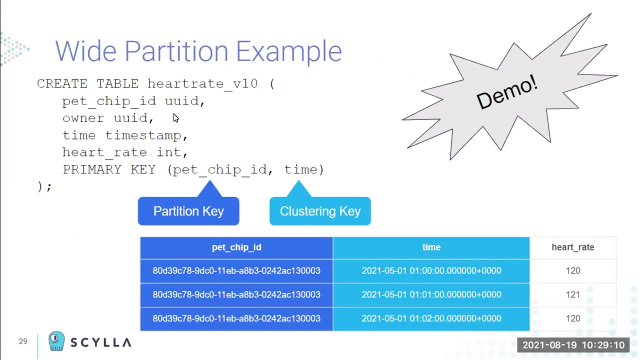 this time and this is slightly more complex. we couldn't do it with that, with the previous table, So supporting this kind of query required this kind of schema. So in this case we have again the pet ship ID, the owner ID. 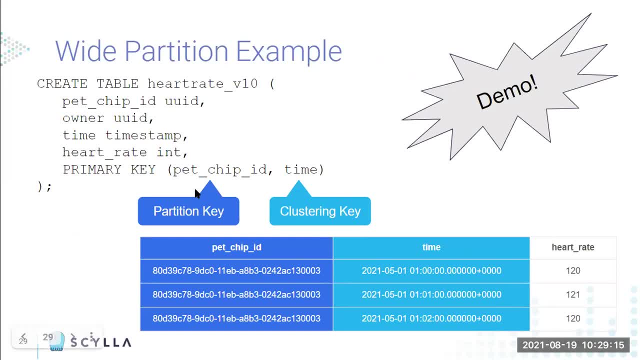 timestamp and the heart rate, And in this case, the partition key is again the pet ship ID. By the way, who thinks the pet ship ID is a good partition key? based on what we've seen before, Is it a good partition key? Raise your hand if you think it's a good partition key. 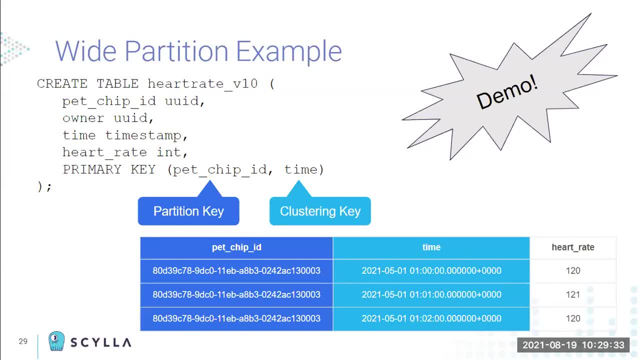 Okay, I cannot really see you, but let me tell you the answer. It is a good partition key because we're using a UUID here, so likely it will be nicely distributed across the nodes. The clustering key in this case- that's a new thing- is a time. 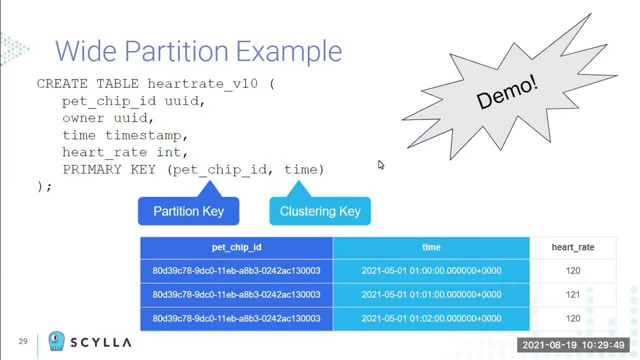 So, on each partition of a specific pet, we have a lot of rows. Each row represents timestamp and a value, timestamp and a value, timestamp and a value. So the clustering key in DynamoDB they call the clustering key ordering key, because it's allowing you to, or it's basically. 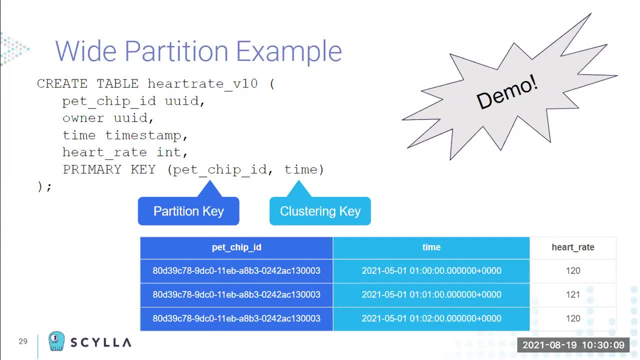 ordering the row in a partition, And the same goes for Scylla. In Scylla we call it clustering key, but it has the same function. Okay, and with that I want to just let me try a quick demo here. 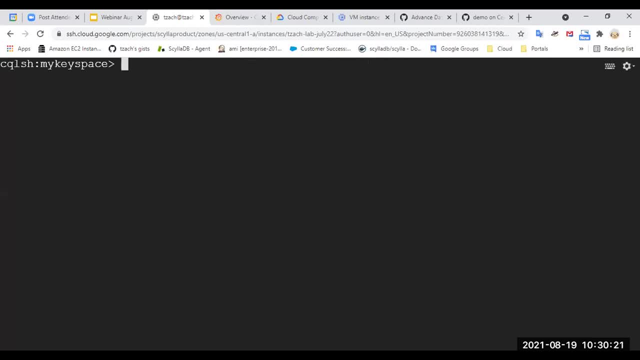 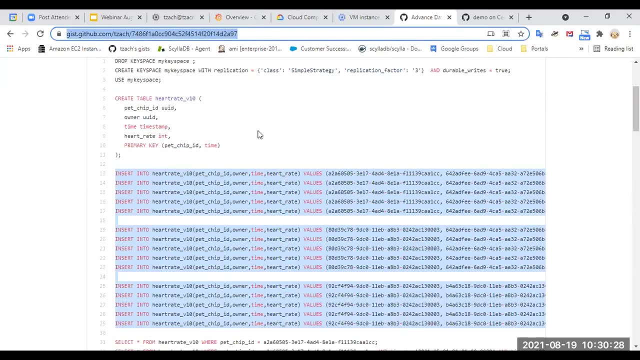 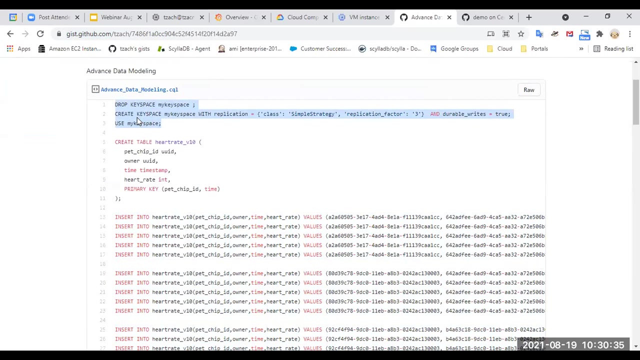 So I'm switching between screens. I hope you can see what I'm demonstrating. And, by the way, I'm copy pasting from a Git example that there is a link. I will share the link after, So let me quickly copy paste. I hope you can see at least some of it. 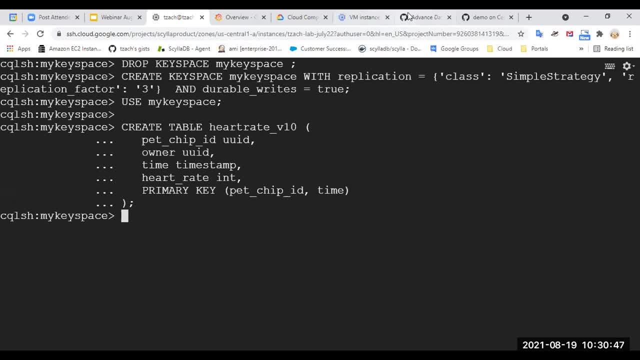 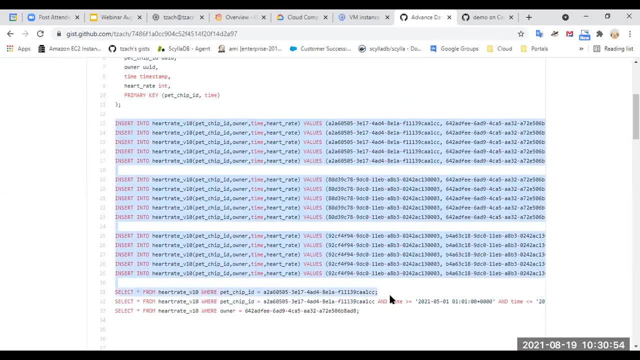 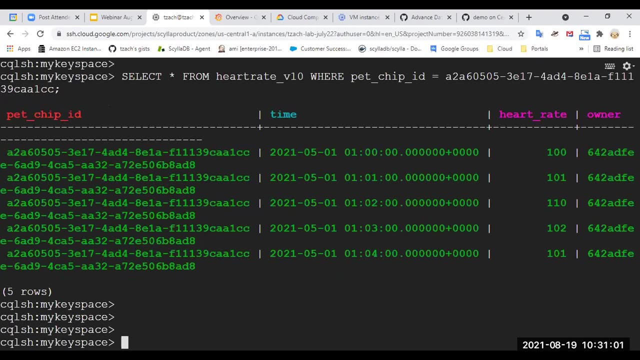 A session without a live demo is pretty boring, and if the demo fails it's even more boring. So let me insert a few heart rates here and then do a select. Okay, so you can't really see the difference, but I insert. I use insert to insert a bunch of. 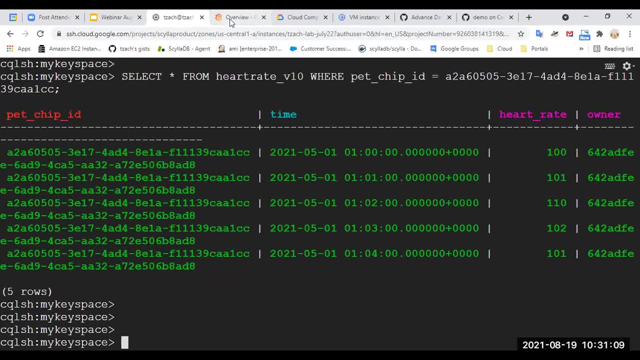 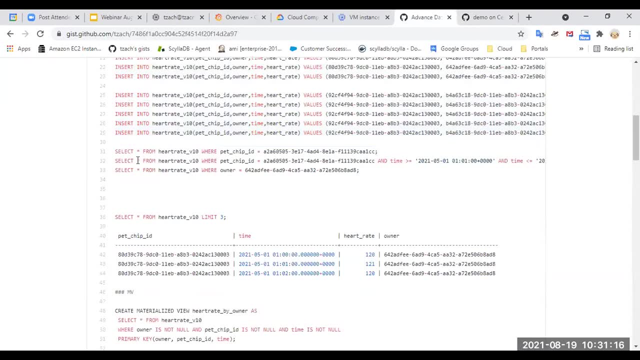 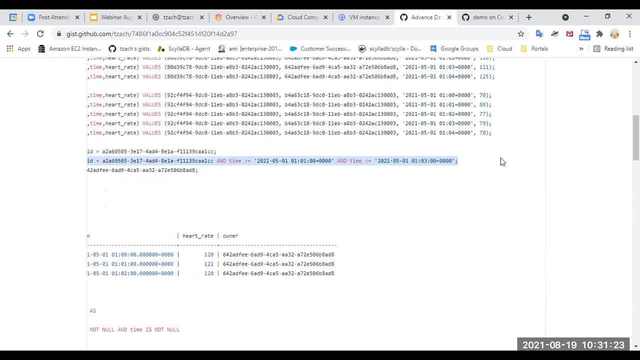 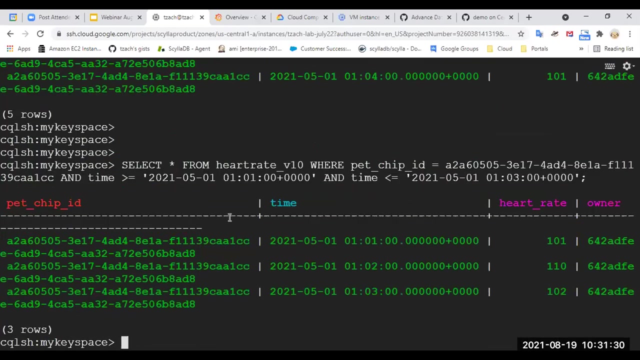 dummy part rates. No, dog was actually used in this demo, so don't worry. And I can also run a query like the one that I presented earlier, which is select, Select with the time range. Let me- Okay, I hope you can see at least part of it, but I did a select. 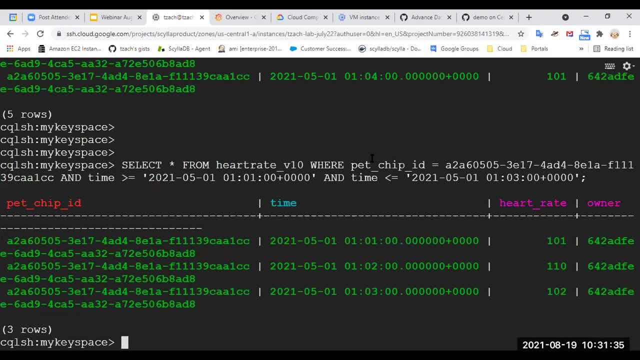 with the workloads of PetShipID equals a specific time And the time range is very, very efficient. Why it works very efficiently. The partition key already limits the database to a specific node, or three nodes in the case of replicas. So it's already fast And the time range is done on a specific partition. but the partition is 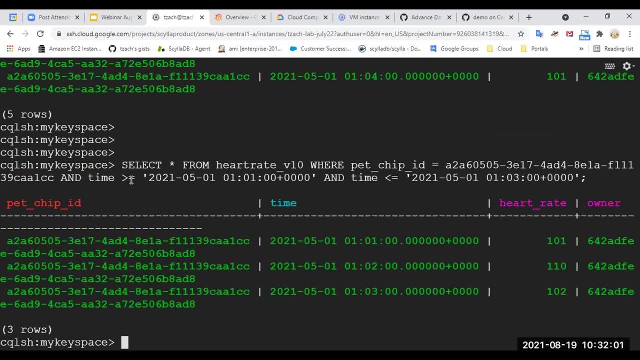 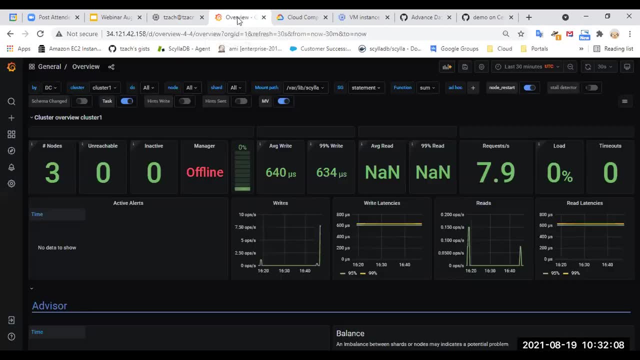 already ordered by time, because time is the cluster key, So it's very efficient to do a query like that and that will practically be less than a millisecond. we can actually go back to the monitoring and this is the Scylla monitoring dashboard, available in Scylla cloud but also in Scylla, open source enterprise. it's it's an open 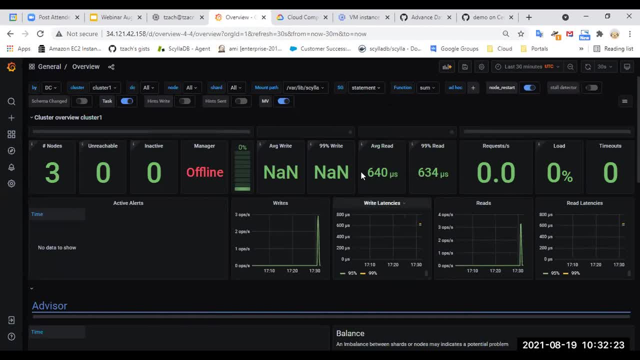 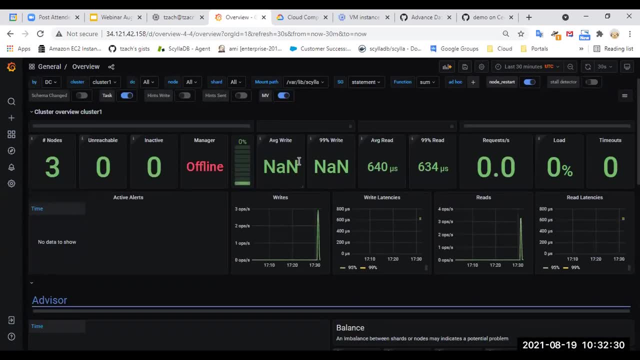 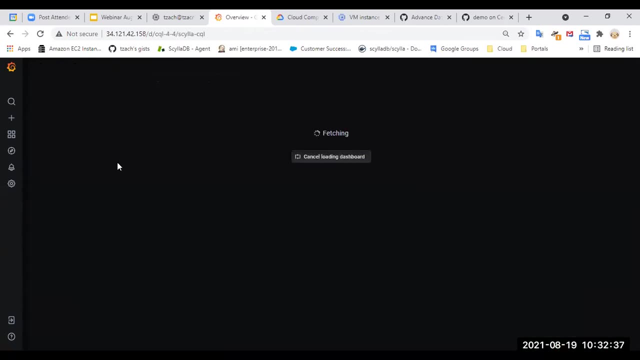 independent open source project. I don't have a lot of value here, so some of the value are not presented. this, that's a overview dashboard. okay, let me quickly jump to another dashboard. here we have like a few of those. there is a CQL dashboard. it can be useful to check out, read and write. 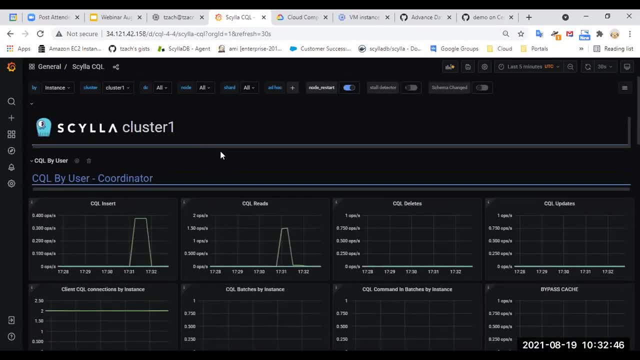 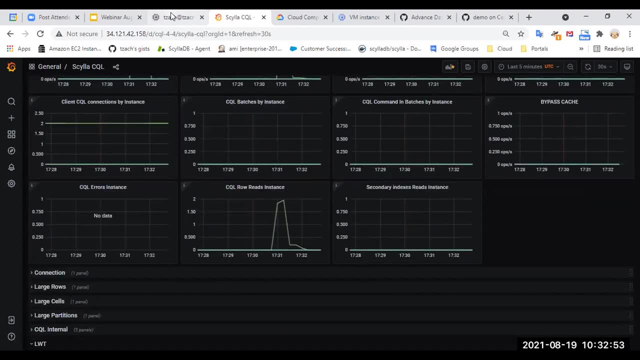 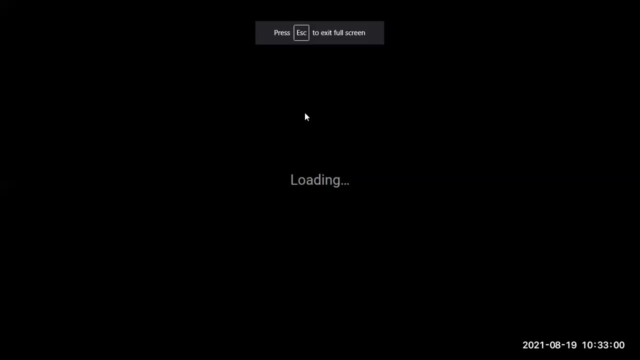 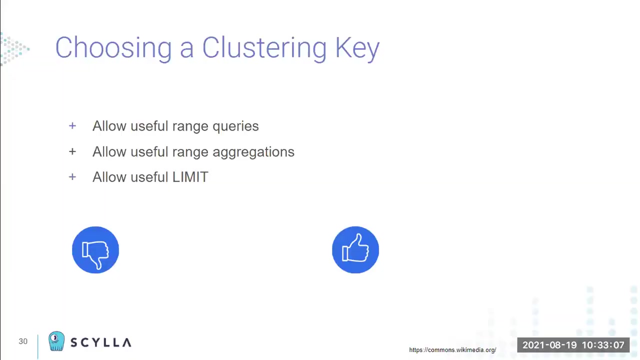 and, okay, I don't have a lot of data here, so the latency will be very, very long, but it's not as representative. okay, let me go back to the presentation and maybe we'll demo something else later in this session. so what will be a good clustering key? so we already agree what is a good partition? 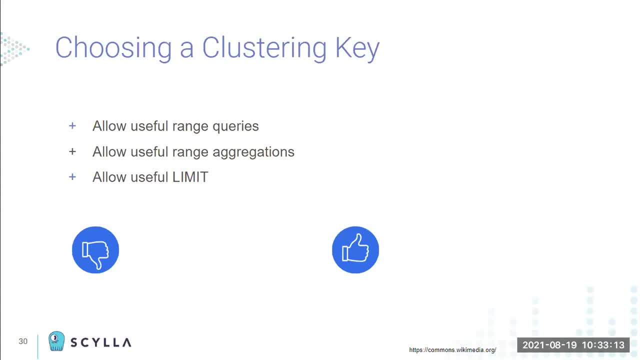 what is a good clustering key? again, the clustering key, the term, the order of the row in the partition. so we want to order it in a way that is useful for your query. I already mentioned, first, if you define what is the core of the application and second, you want to model it. 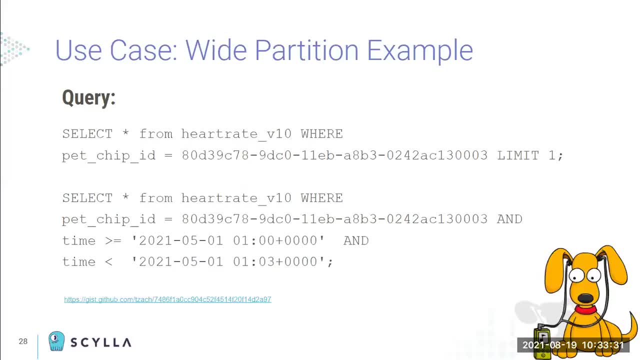 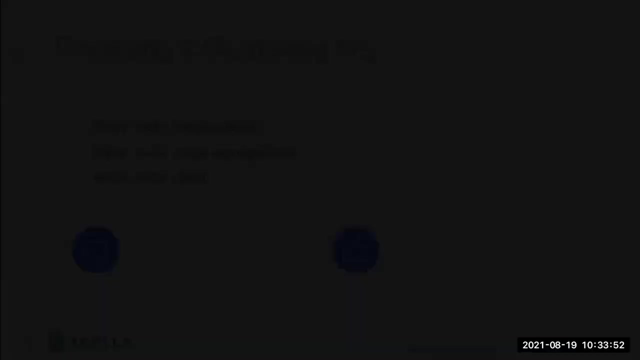 so in my example, just as a reminder I started with, I want to do this kind of query. so in a partition key I want to either get the last value or the value between in a specific time frame. so using time or timestamp as the clustering key make a lot of sense. it's not true for all cases. 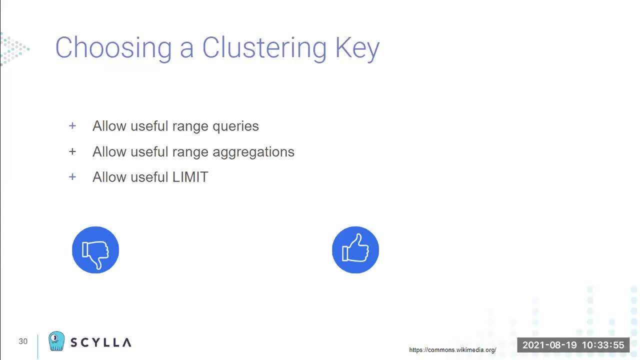 and in many cases we actually don't need a clustering key. so in my first example of just keeping a data store of the pets and the pet's name, I don't necessarily need a clustering key. if I don't, you don't need to use it. you actually don't need to use it. you actually don't need to use it. 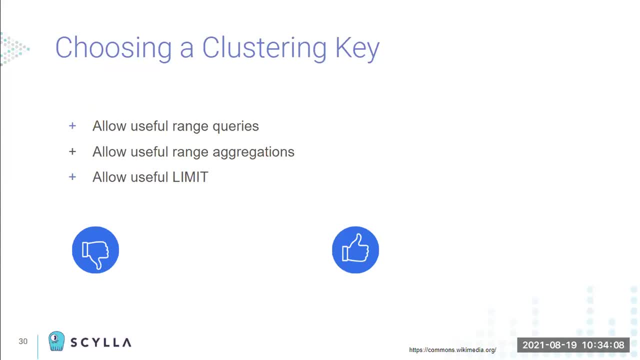 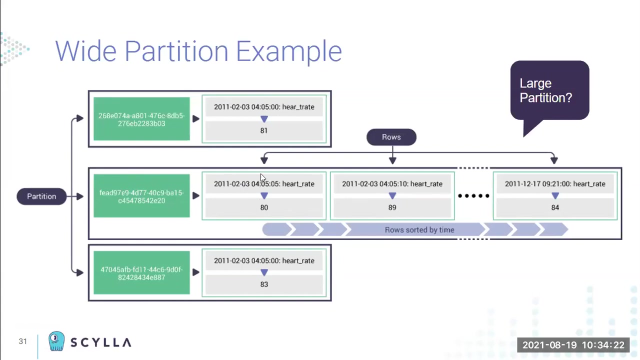 actually, it's better not to use it if don't. don't force it, but if you do want to order order on a partition key, use the clustering key and this is how it would look like. so, for a specific partition key, we have a lot of rows. each row, all the heart rate and a value: heart rate and a value. 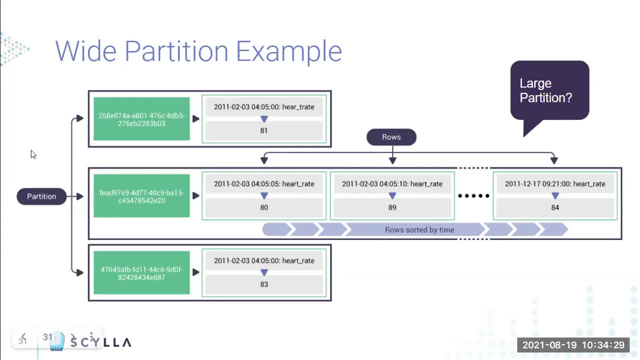 and I'm sure that some of you already think: hey, how many, how many row can you? can you fit into one partition? yeah, so that's a good question. and okay, let's say in this slide: that's a good question, and if you're putting a lot on a lot of row on the same partition, at some point you will get to a 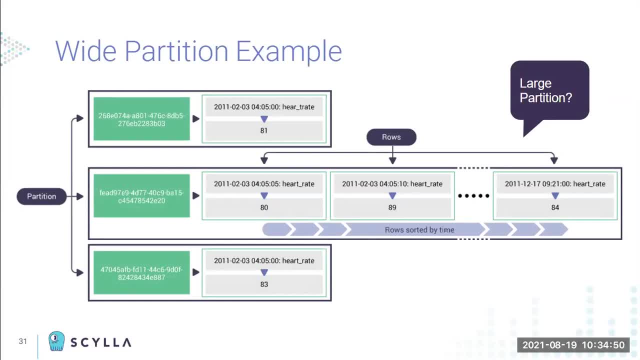 large partition situation because you might have millions and millions of row in the same partition. is it a problem? so two years ago I would say yes, but. or three years ago, but since then we did a lot of refactoring Scylla. that basically solved this problem. so you can have me easily have millions and millions of rows in the same. 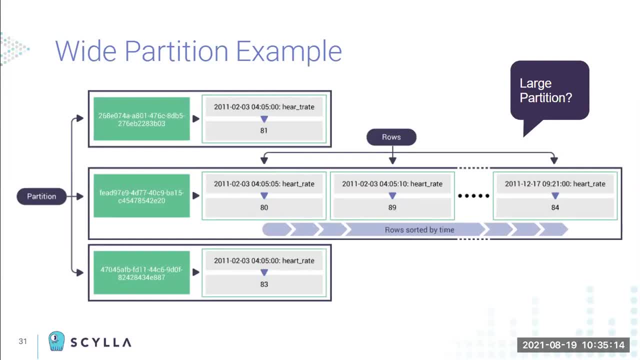 partition and won't have a problem. and recently we've seen on production a partition of 200 gigabytes, which is used to be considered huge but it's supported. you do want to be careful about a large partition becoming hard partition, so if all of your traffic is going to the same partition, 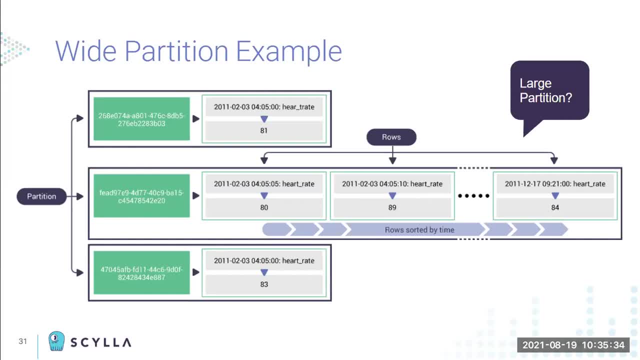 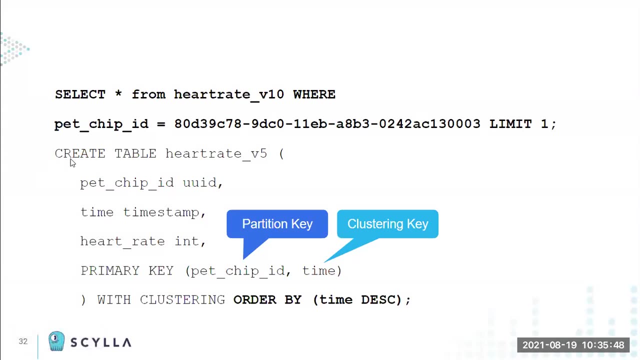 you might have a problem. so the general recommendation is: to have a large partition is not to have huge. huge partitions and millions of flow will be supported. if you can even go below that, usually it's better, but it's depend on the use case it is supported, and so we- we've seen the 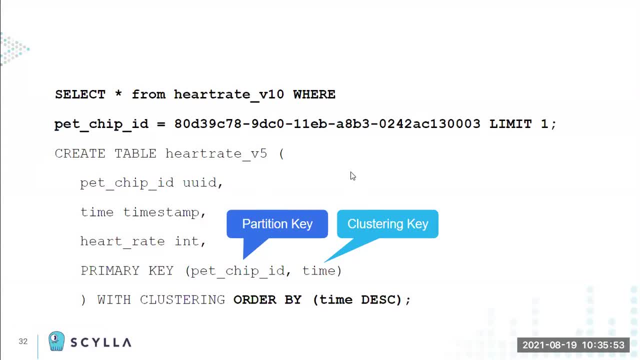 partition. we've seen the clustering key. when you set the clustering kid, it will also also set an order of the clustering key: ascending or descending. what to choose, choose based on what you query for. so if, in our example, to query the latest value every time, so ascending makes sense because i can just put limit one and 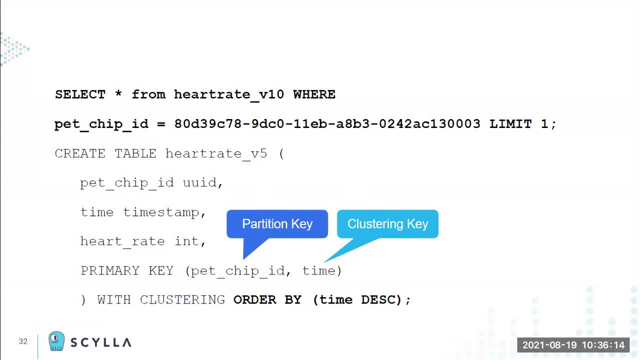 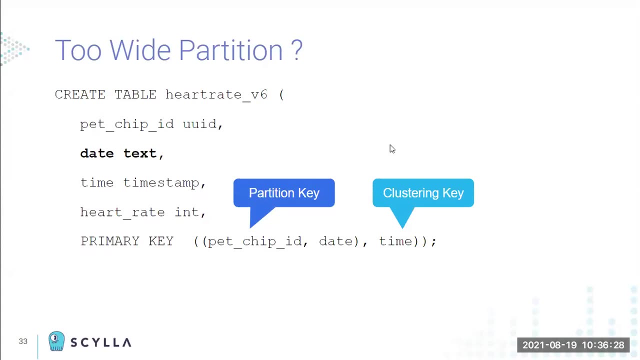 have it very fast. if it's the other way around, choose descending, you can always query on the reverse order of the classroom key, but then performance will be not as good. so it is possible, but you will get some performance. it in a case that you think you you got a too wide partition. 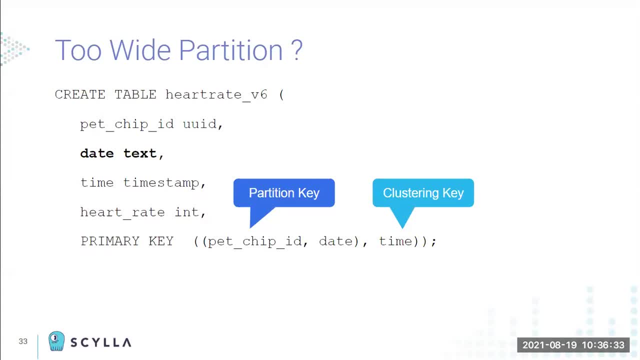 as i mentioned earlier, there is a way to handle that, and the way is to create a component partition key. what is a component partition key? we are basically adding elements to the partition key, in this case the date. so if we used to have, like, a huge partition key holding all the information of 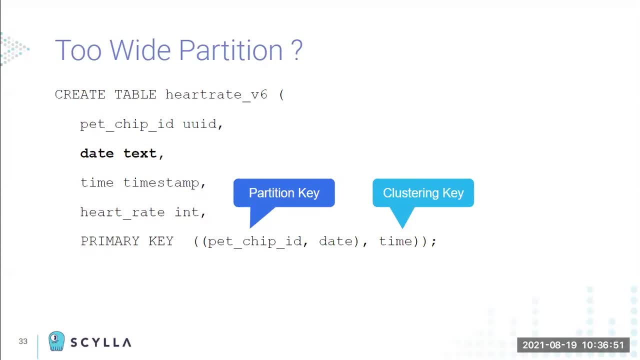 all the time information of specific pet. now each partition hold only one date, so there is pros and cons to this approach. the pros that yeah, yeah, yeah, now you have a limited number of uh of all per partition, basically the number of seconds on a day in this example. and the the cons of this approach that if you want to query all the 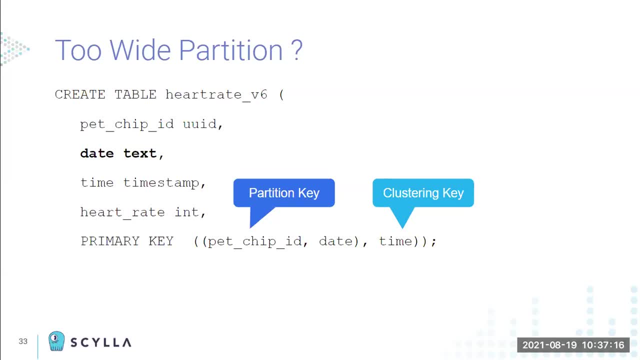 information from all the days. you have to query more than one partition, and so it's a little bit more work from the application side. in return of that, that, you don't put a lot and a lot of that on the same partition, and of course it's. can it can you can use other fields that 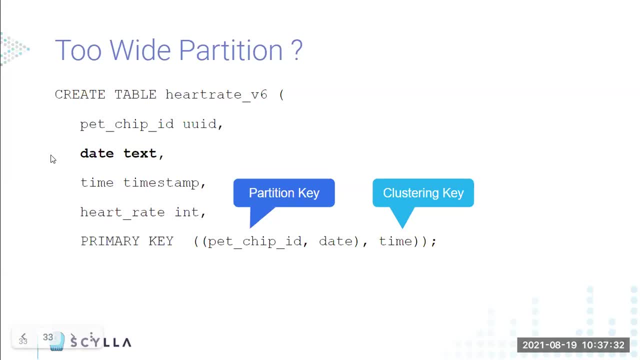 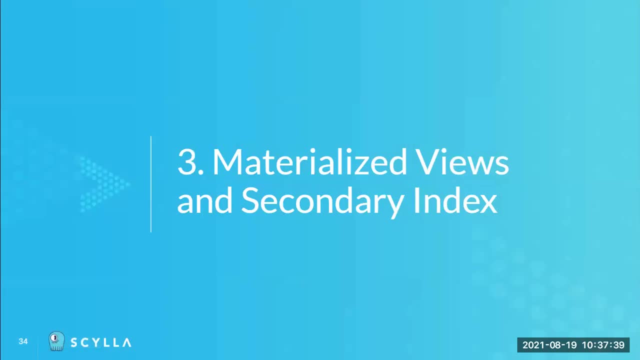 you have a lot of partitions, so this is just an example. the idea here is breaking the partition to smaller partitions. okay, so i hope i i gave you some insight into a partition key and and the classroom keys and this. the last item i want to touch on this session is materials view and probably not going to get to. 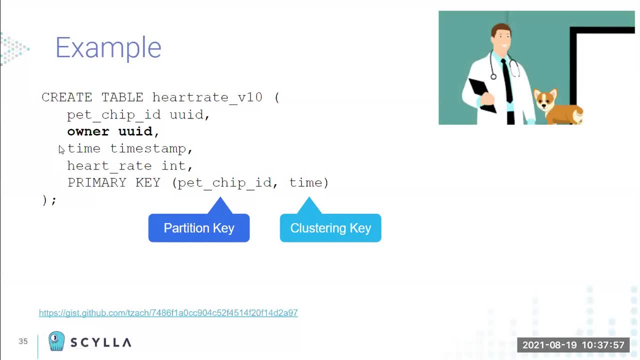 the secondary index. so what? what is the materials view? the? the view is a context of the data, that's. This concept actually exists in many databases. I want to give you the Scylla or the NoSQL variant of it. So let's say, going back to the example we had before, 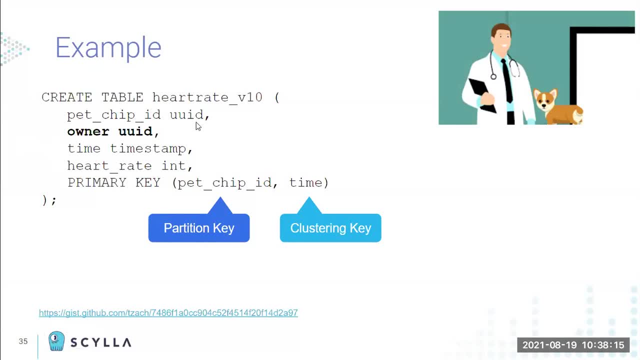 So the example we had before, quick reminder: the partition key was the pet ship ID cluster key was time and we had the owner ID. Till now we just ignore it. But now I want to actually query by the owner ID. 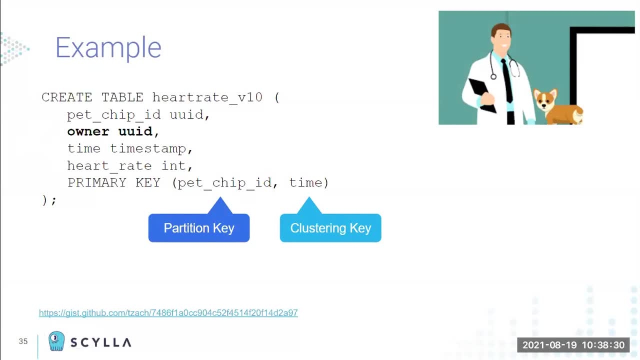 I want to, for example, have the all the measurement of the specific order. So this is actually not. it's not a partition key, It's not a clustering key. So we already know it's not going to be efficient. but on some cases, my application. 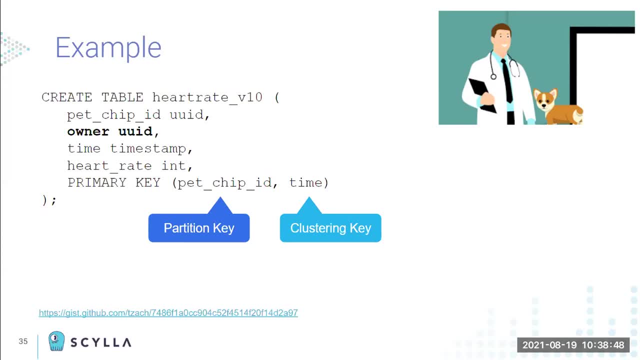 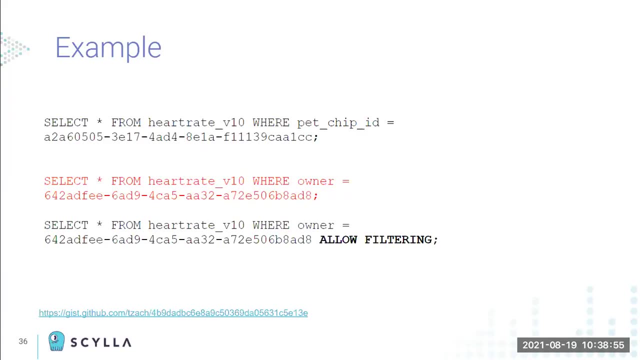 the application developers say, hey, fine, you created the schema. Now I want to use another column as a key. So what will you do? So if you naively try to select using the owner is equal, you get an error back saying, hey, this is not supported. 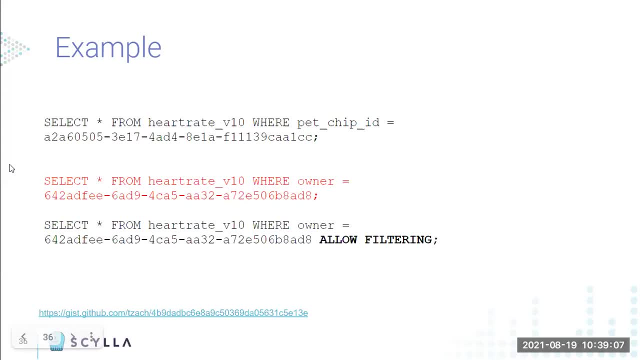 You need to use allow filtering. Why is that? Scylla try to warning. If you, if you want to, and you actually force Scylla to run this code with allow filtering, behind the scenes, Scylla will have to scan all the nodes for all the data. 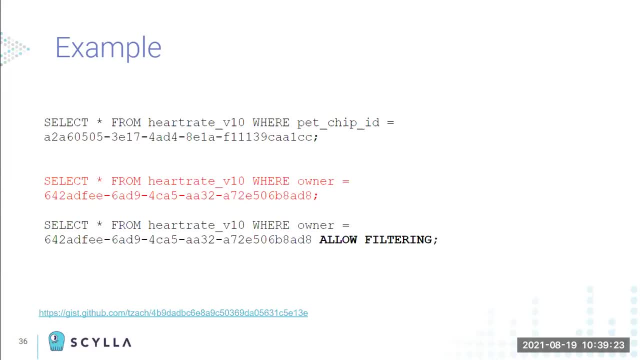 and find the specific owner and send you back the result. It will work, but the performance will not be as good, And if you have billions and billions of row, it's actually going to be bad performance. Maybe, maybe you don't care. 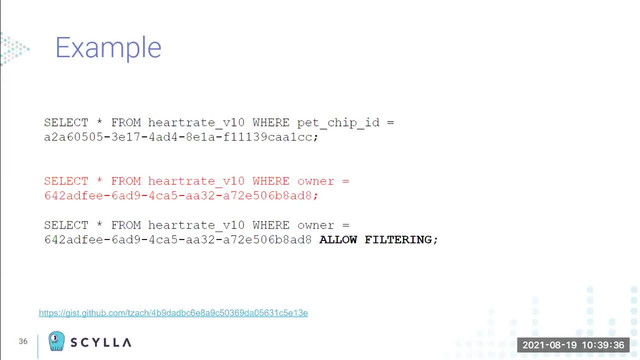 Maybe it's the right option. I will explain later why it makes sense in some cases. But if you want to have a very quick sub millisecond response for this query, you won't get it with allow filtering, And this is where we introduce a material view. 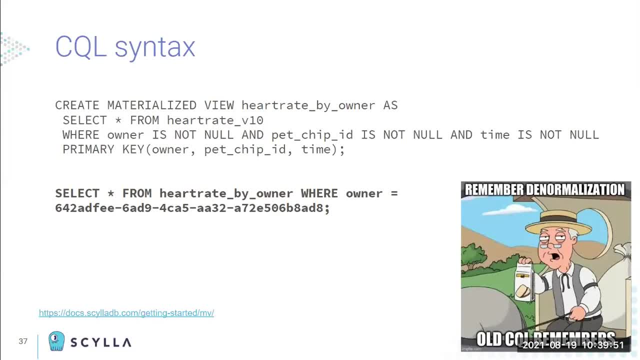 A material view. you can think about it as denormalization. people that work with NoSQL are used to denormalization. denormalization is basically take the same information and put it twice, insert it twice in the database, every time with a different key. 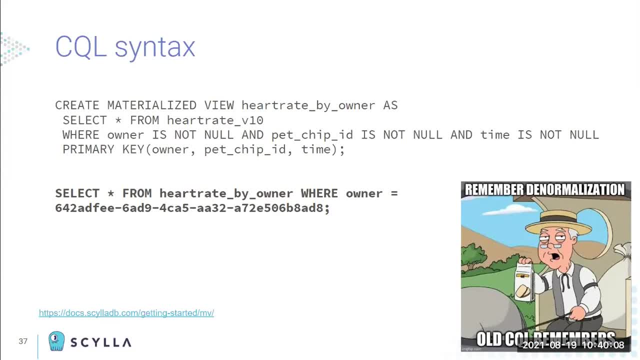 so that you can still do that with Scylla. sometimes it's useful. the problem with that is that you have to manage the synchronization between these two tables yourself, and it can be extra work that you don't want to do. so you create a materials view. 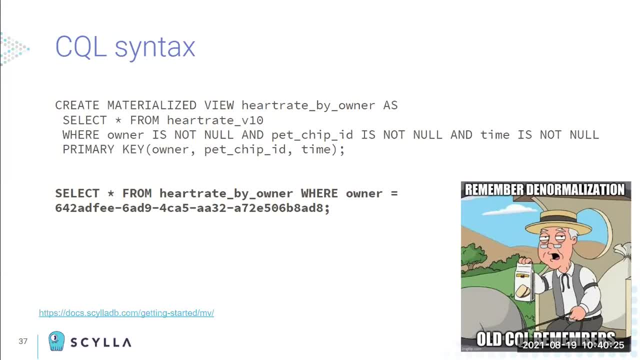 materials view is automatic denormalization. so Scylla will create another table for you with the same data, with a different key, and synchronize between the two tables automatically. so if you delete one here, you delete here, update, update and such, and this is. I don't want to spend time. 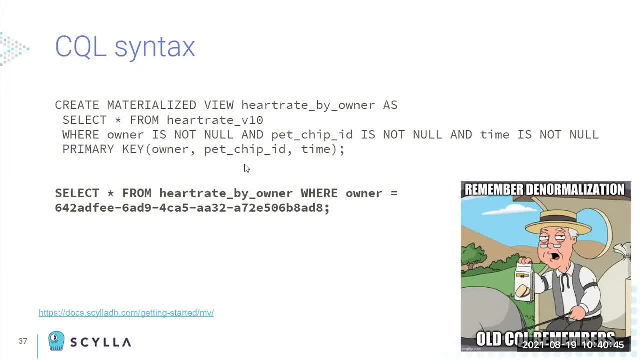 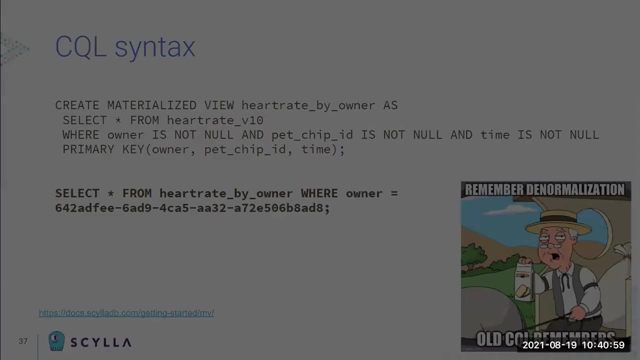 on the syntax itself. but once you create the view, you can use it to select by the owner, because the owner is the partition key in the view. it's not the partition key in the base table. so that's an efficient way to query by a column which is not the partition key. 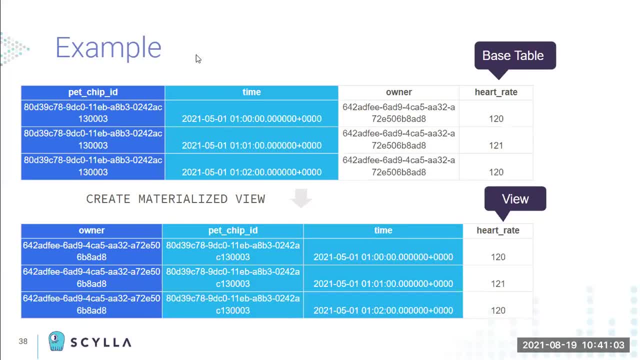 and this is how it would look like. you can think about it as a transformation of the original data to a new table. now, keep in mind this table will not necessarily be located on the same nodes, because it has its own partition key. partition key leads you to the node. 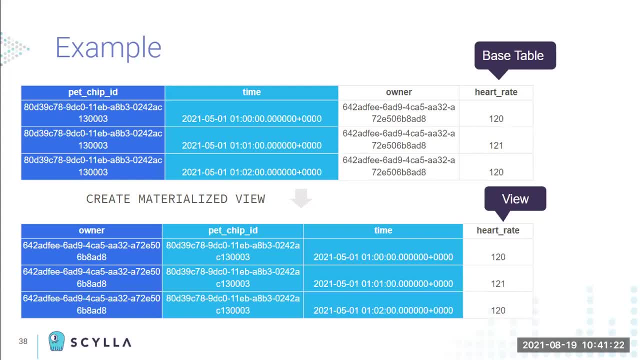 so the view in the base table will not be located on the same nodes, so the view in the base table can be on separate nodes. of course, Scylla takes care of that. you don't need to worry about it, but keep it in mind. it's also similar to denormalization. 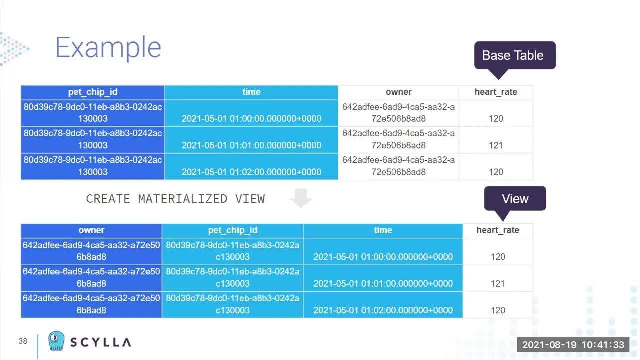 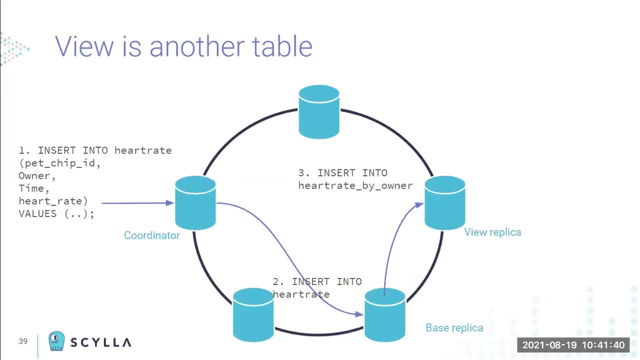 you pay for it by storage, so you are keeping the same information twice on disk, so it has its cost. this is how an update to a view will look like. Scylla will first store the base table of the information and then update another node with the view information. 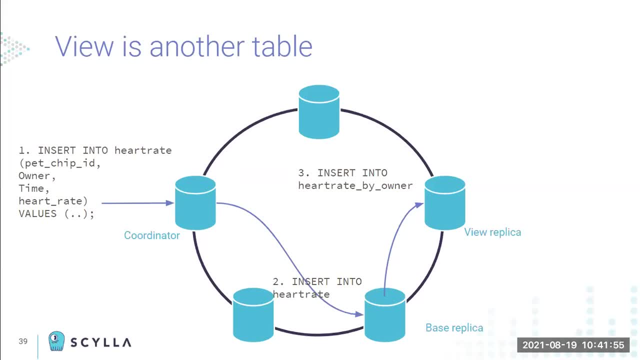 and now this is actually a simplified diagram because in practice there are usually three replicas, both for the base table and for the view. so there are more errors and more messages and more storage, and that's the price that you are paying for keeping the same information twice. 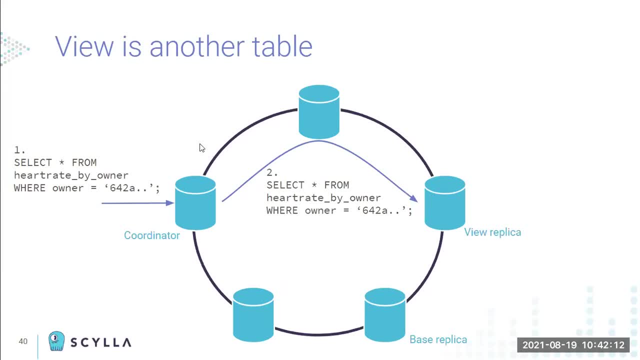 the read from a view is actually pretty efficient because the view already holds the data and the coordinator can go directly to the view and fetch the information from there and the view can go directly to the data. by the way, in practice, usually the coordinator is already one of the replicas. 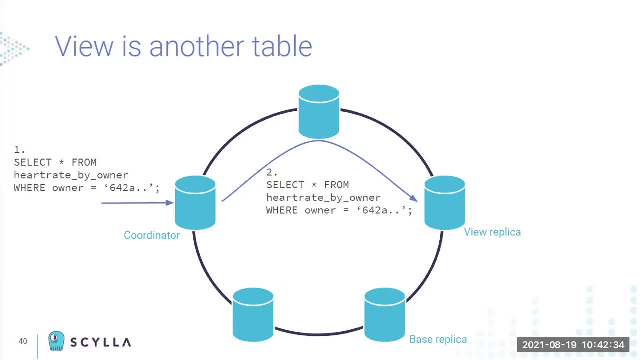 if you are using the latest driver from Scylla or even from Cassandra, the driver tries to optimize the query by going directly to the replica. it's an optimization, so in most cases it will hit and if it misses it will act like it's shown here with the coordinator. 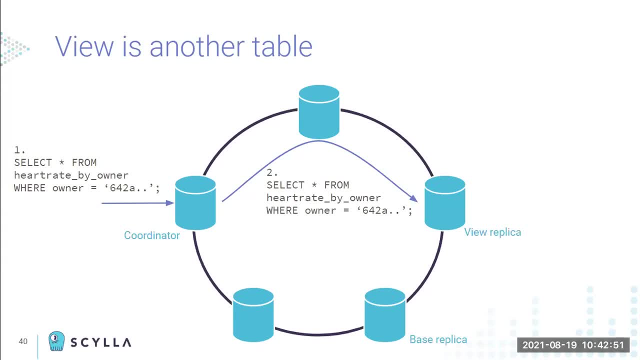 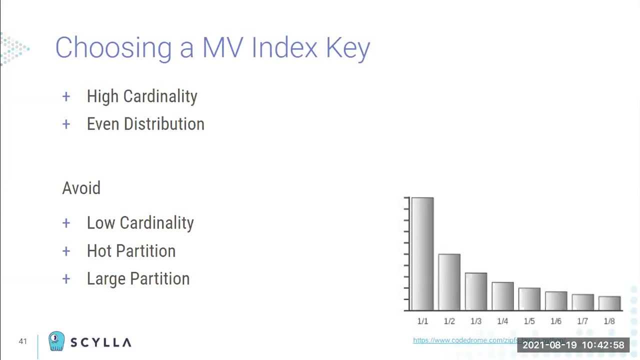 to send a message to another replica, but in most cases there is actually only one message coming to the database: how to choose a good material view index. exactly the same. the same reasoning to choose a good partition key if you try to group a lot and a lot of rows. 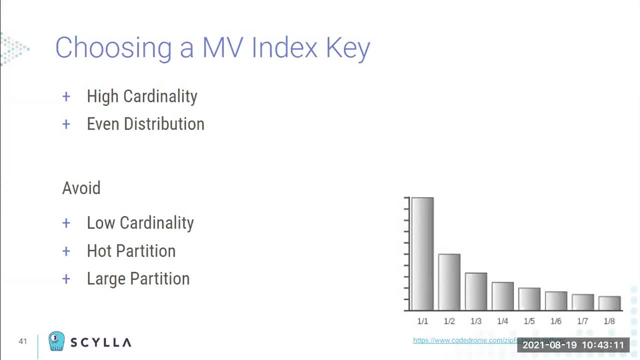 into the same key, you will likely have a problem. so the owner seems to be a good, a good candidate for a materials view index, because there are a lot of owners. but if you choose a good material view index, you will likely have a problem. but if you choose a good material view index, 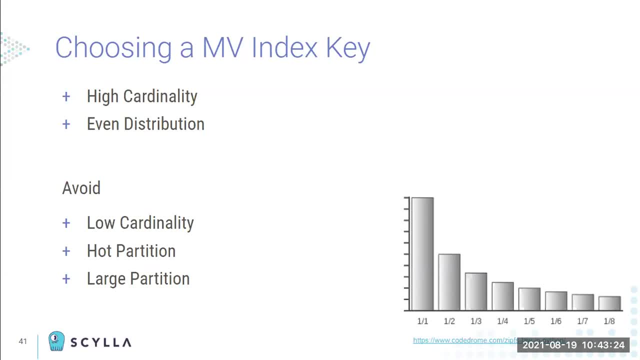 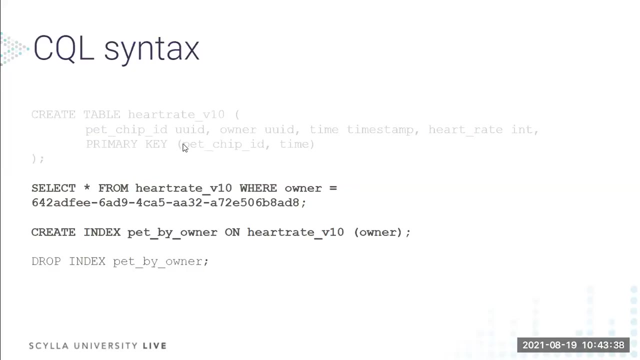 but if you try using something like age or state as a key for the materials view, you will likely hit a problem, as we mentioned before. so it's the same story back again. global secondary index: you can think about it as a syntactic sugar in Scylla on top of materials view. 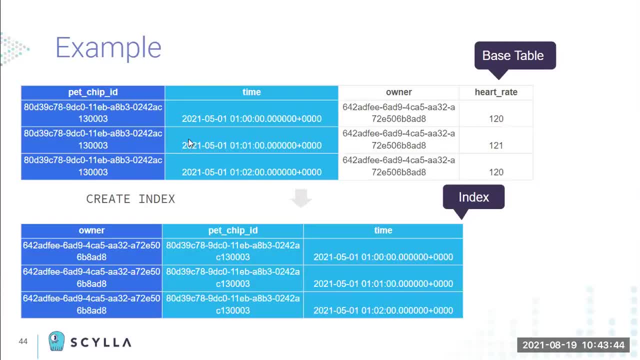 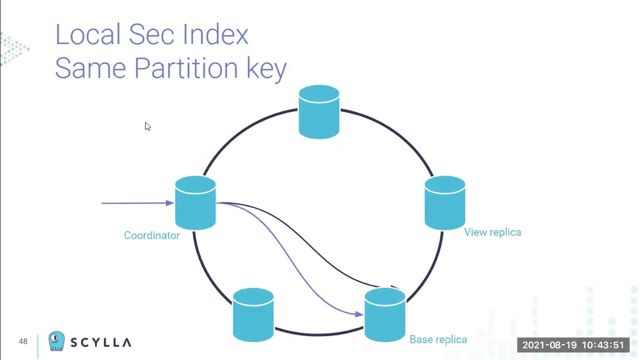 it's have slightly, I'm not going to spend too much time on it. I do want to mention that. two things first, and let's go for other databases as well, for people using DynamoDB. so this should be familiar to you. if by chance or not by chance, 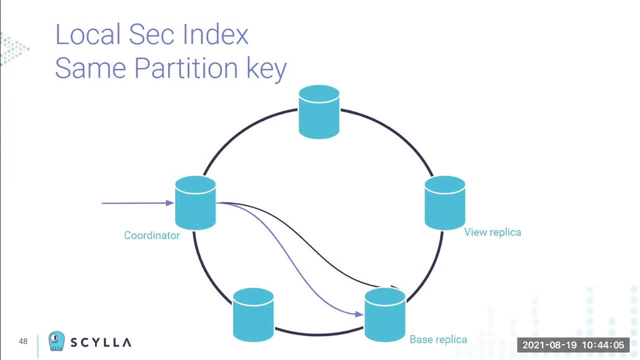 sorry, by design, you are using a secondary index or a material view with the same partition key as the base table. Scylla will optimize the implementation based on the fact that the view and the base table is using the same partition and the data is on the same node. 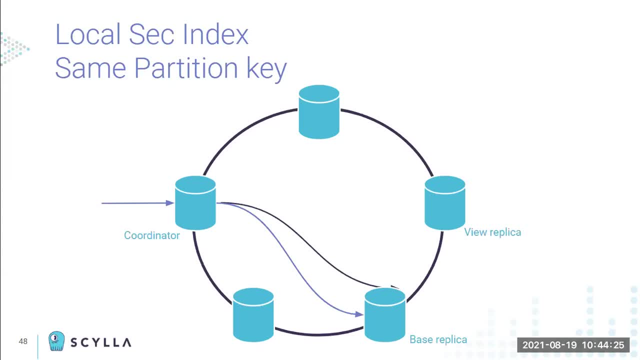 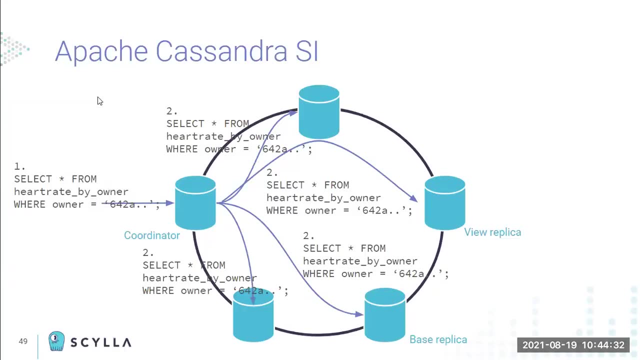 so earlier I mentioned that the view and the base table are likely not on the same node. if the partition key is the same, they will be on the same node. so Scylla, use that for optimization. people coming for Apache Cassandra, Apache, Cassandra- also have secondary index. 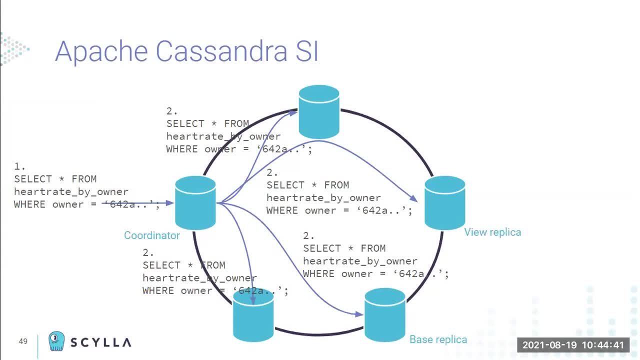 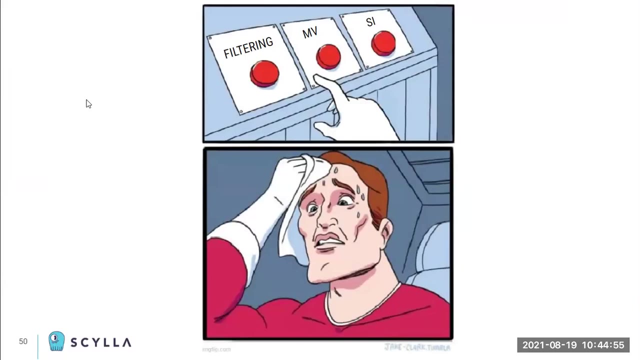 it have the same syntax as Scylla secondary index but the implementation is different. so keep that in mind that if you're moving from Cassandra to Scylla and use secondary index you might see different performance characteristic. so we actually seen three different way for query. 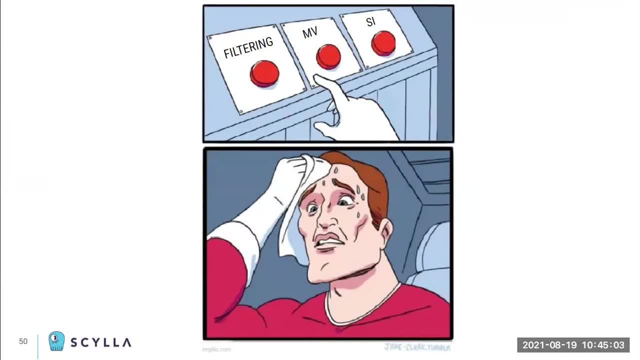 Scylla table not based on the partition key. so the best way. and then the highway or the main road if you will use the partition key and you almost guaranteed to have sub millisecond result. but if you want to query on a column which is not a partition key, 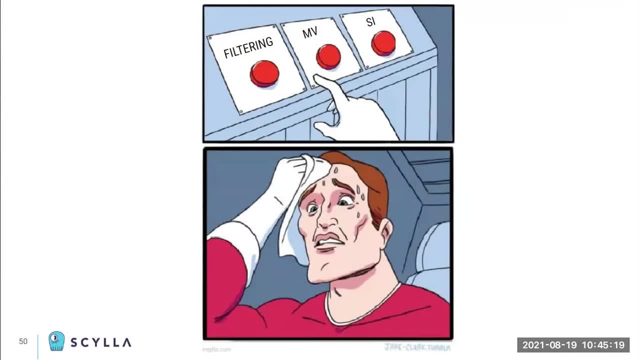 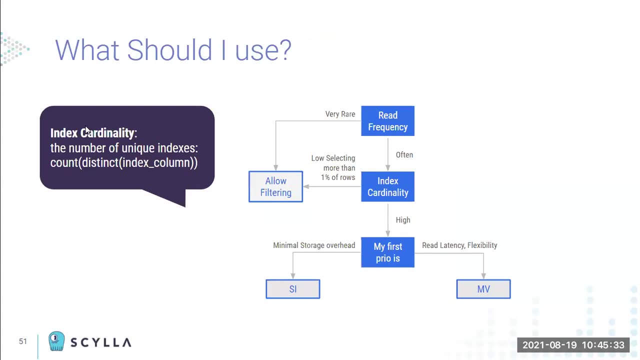 you have three option. one is using filtering, which is basically a full scan of the data. second, material view, secondary index, which have slight difference that I'm not going to cover here. so think about it as the same, roughly the same option with this scope. so what you should use. 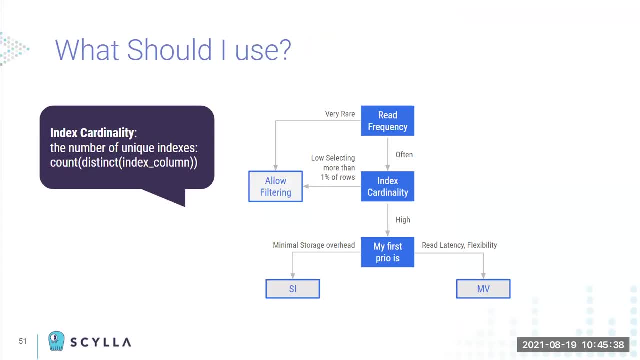 if so, like the rule of thumb, if this query is very, very rare, it's something that we are running ad hoc, maybe once a day, and you don't care as much about the latency of this query. just don't care about the latency of this query. add an index, just run with allow filtering. yes, it will load the data, it will do a full scan, but 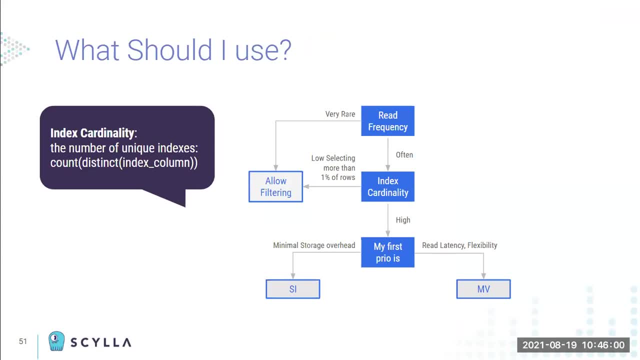 maybe you don't care as much. if you do care about latency and you want this product to be a sub second, then do create a materials view. and again, i'm not, i'm not going to cover the differences between the secondary index, under whose it's pretty much the same. 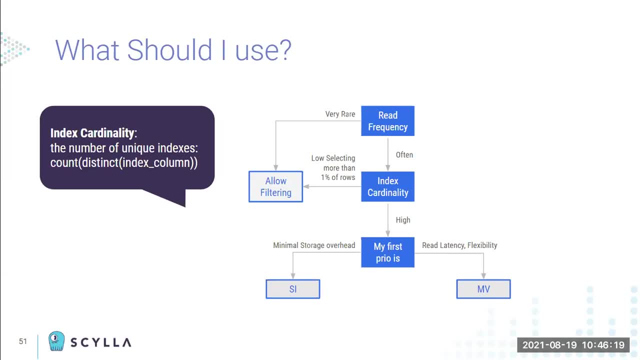 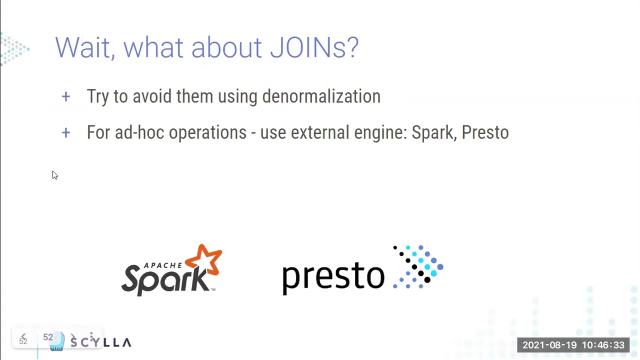 and, by the way, you have a fourth option of just denormalization data yourself, so you can always insert the data again from your application, but then you have to manage the synchronization yourself. in some cases it does make sense. and so, last but not least, what about jones? so let's say: 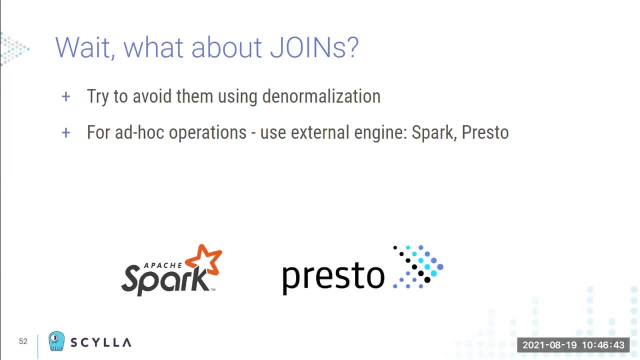 so far i saw pretty simple queries and it is the sweet spot of json. so let's say: so far i saw pretty simple queries and it is the sweet spot of json. so let's say, so far i saw pretty simple queries and it is the sweet spot of. 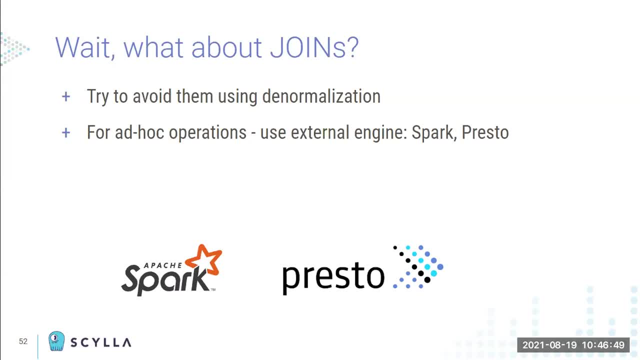 scilla to worry by the partition key, not doing join at all, but in some case you do need to do something like that, and so what can you do? so syllabi itself does not support join, but you can use third-party tool like presto or spark that work very nicely with scilla. 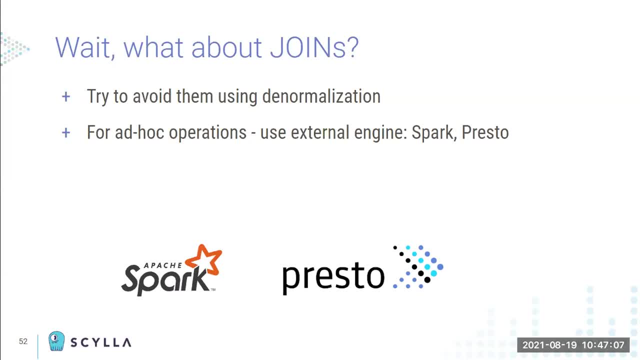 of course this tool can do a lot of things: transformation and and complex scoring. just keep in mind that likely this query will be translated to full scanning the database. so keep in mind it won't be very efficient in most cases to use this tool. but again, if you don't, 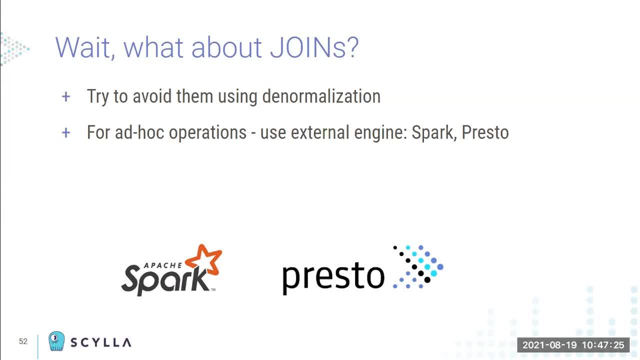 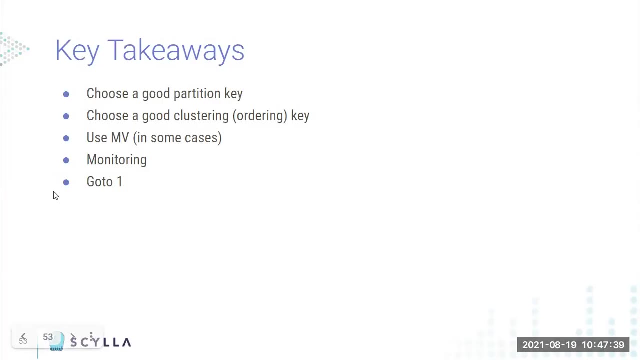 in many cases you have, like a specific query that you need a sub millisecond response time, another query which you don't really care, like analytics, that can run at night for hours, and then this tool become very handy. so we are almost done. so what are the key techniques? 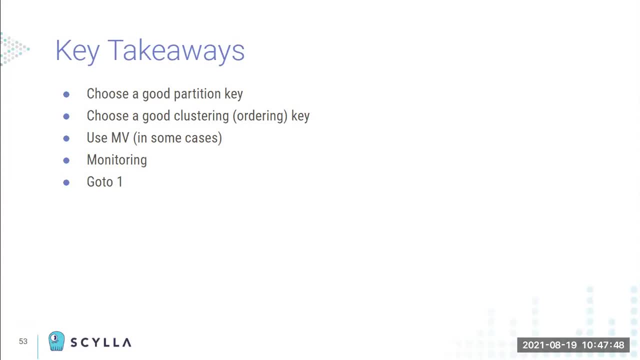 that you need to take away for from this session. the first one: choose a good partition key and if you remember just one thing, is this one, it's the most important. a second: if you need to choose a good classroom key, if you don't need a classroom key, avoid it. third is, in case you 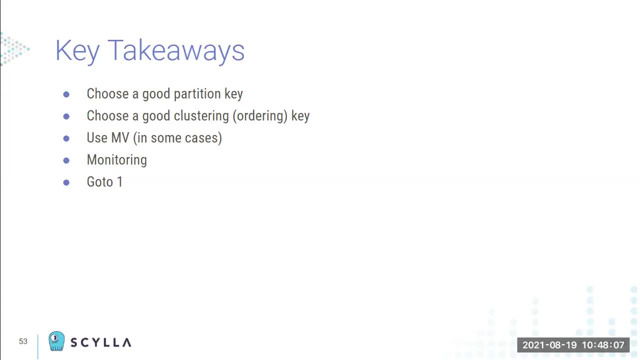 want to query by a column which is not the partition key, and i want it to be very efficient: use materials view. the next one is monitoring. so so monitor, monitor, monitor, don't on a general don't. don't start a benchmark, don't test a new database without a very good monitoring tool. in scilla, we have this open. 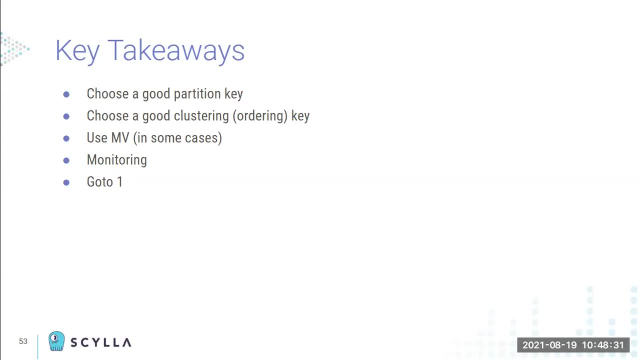 open source monitoring stack, other tool, have other monitoring tools, use them, otherwise you're basically blind and i can tell you that if people are in the open source or enterprise project, are calling support, asking them for help, the first question will be: please show your monitoring data and last go world one. it's an iterative process. 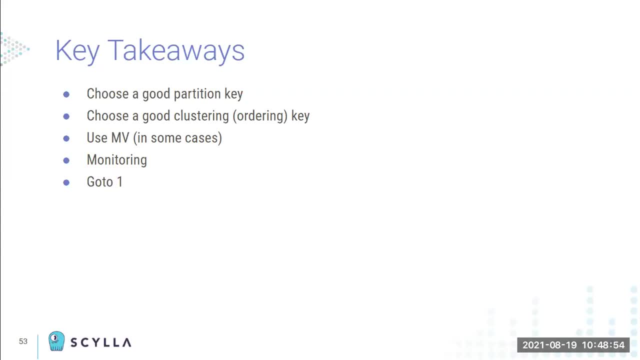 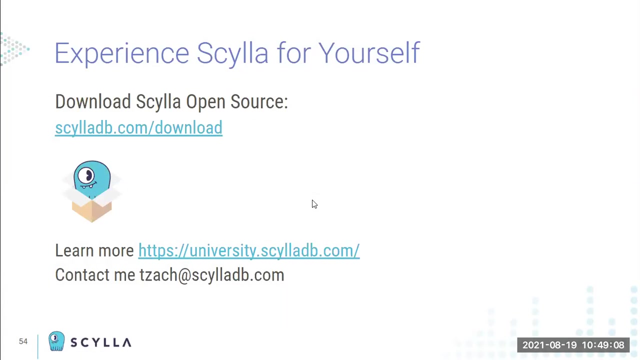 and the schema that you created on day one will probably going to change on day 100, simply because you don't know all the information in advance and sometimes that's a change. so if you want to take sita for a spin- i already mentioned sila cloud- you can also download cinnamon, run it and docker and such everything that i say on this. 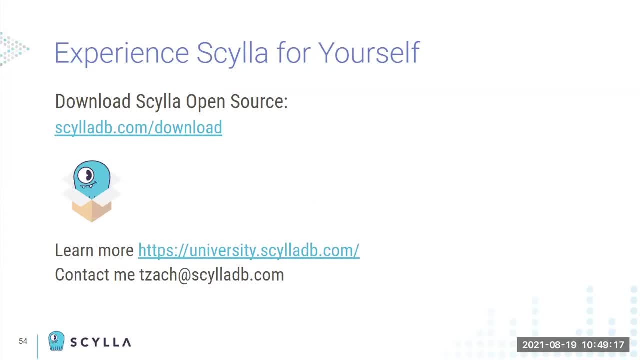 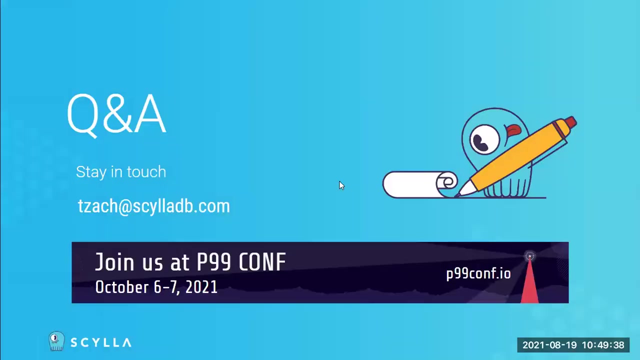 session and much, much more is covered in Scylla University, which have a lot of interactive, cool session there. Go for the data modeling basic and advanced data modeling session for a similar information to what I presented here, but in much, much more details and exercise a really cool site. so check it out. and by that I will switch to the Q&A. 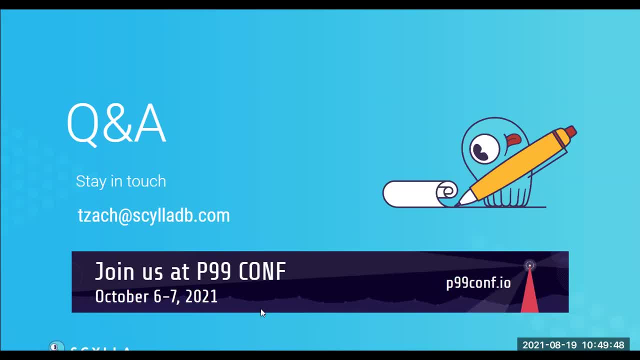 So what is the? I'm reading in a random order. so there's a question: what is? what is tail latency? Tail latency, or sometimes p99, is actually a latency. you, in many cases, you, you're not interested in the average latency for the quarry. 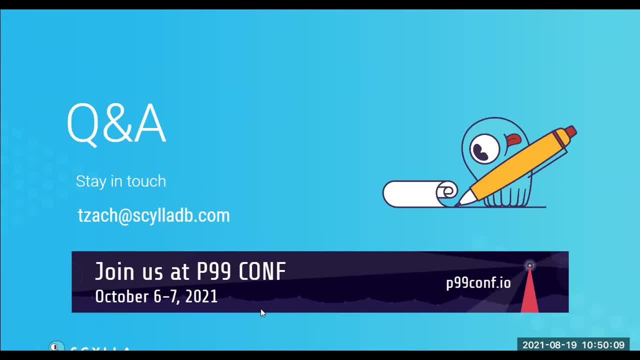 You're interested in the worst one percent of the quarries because this, this one percent may affect the entire latency of the quarry. You're interested in the worst one percent of the quarries because this, this one percent may affect the entire application. so this, this is what they call the latencies, the higher percentage of the latency. 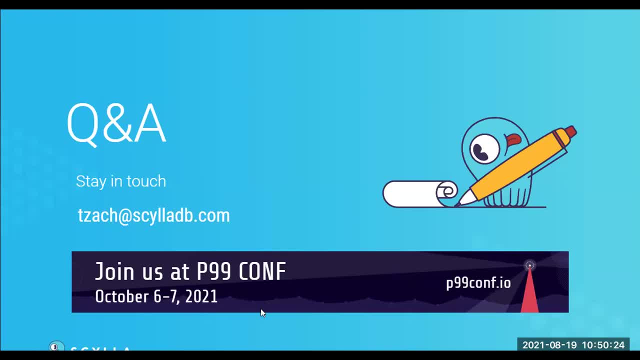 95 or 99. if you're talking about p99, it's the worst one percent of the latency, and this is usually what you need to check, and this is, by the way, what Scylla excel at. so the monitoring, the monitoring stack that I show earlier, do have a dashboard for for the p99 latency. 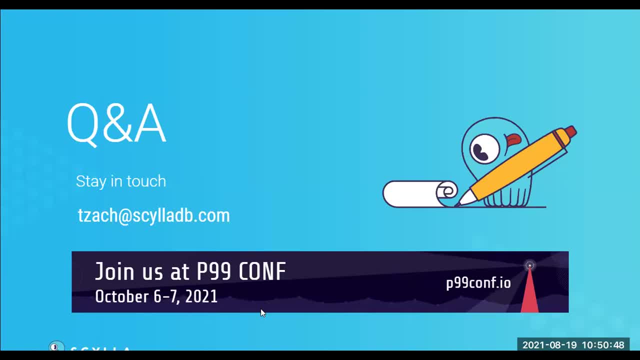 Okay, looking for for other question: is there a way to do a poc on a single node? So yes and no is a quick answer. so, depending what you want to test, if you want to test a functional quarry, like just to test if your quarry is legal or not, working or not, yes, use. 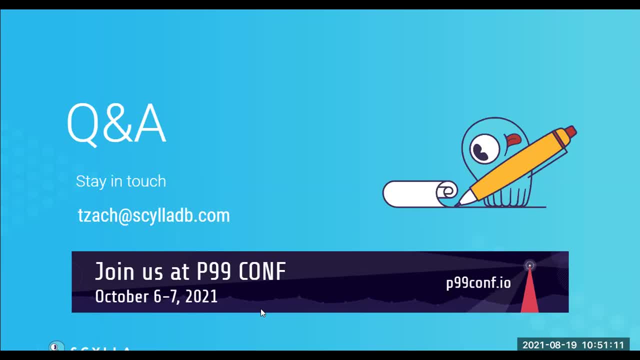 one docker instance on your machine, it will work if you want to test performance. it's not realistic. it it's not realistic because the production database will always be at these three nodes, and so testing it on one node doesn't make sense. you are losing all the communication between the nodes. 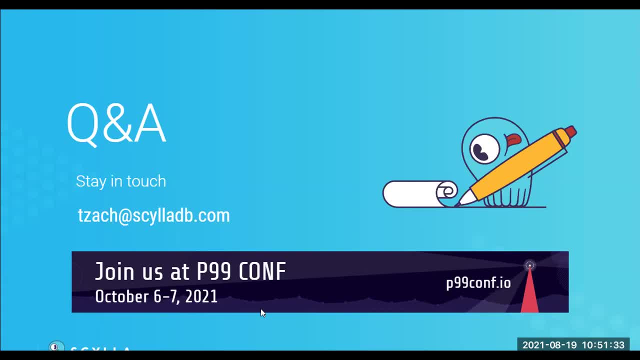 so I would recommend go to AWS, go to Scylla cloud or set up on your own, but don't test it on your laptop. unless you're looking for functional testing, then it's fine. Okay, other question regarding the DynamoDB API. so yes, in this session I mostly gave example from: 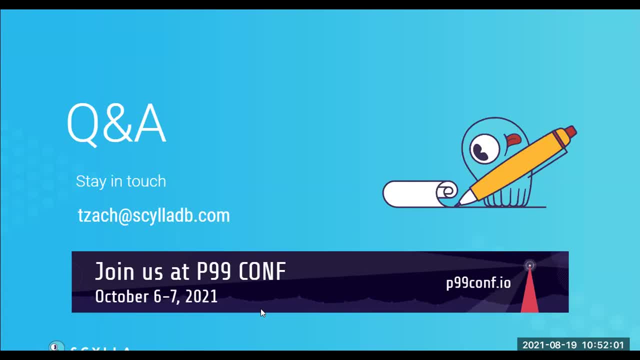 the CQL, but I mentioned at the start that Scylla is compatible both with Apache, Cassandra and DynamoDB. DynamoDB have its own, a different API, but roughly most of what I mentioned apply for both for DynamoDB and serve with DynamoDB API as well. You need to choose a good partition key. 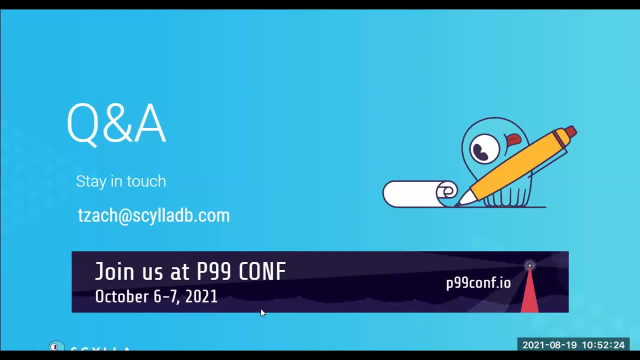 and you can use multiple tables, but the partition key is is the most important. selection and DynamoDB API also have this notion of both partition key and ordering key, or clustering key, if you will. Last question: can we use ScyllaDB to capture telemetry data of millions of data? Yes, you can use ScyllaDB to capture telemetry data of millions of data. 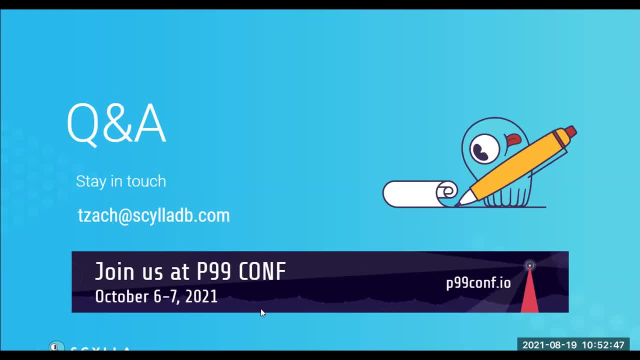 Yes, that's the exact same example that I gave before. Should you put all of the data of one sensor on the same partition key? Again, yes and no. So depending how many data points you have per partition key and depending what query you want to run, on some cases it does make sense to put everything on the